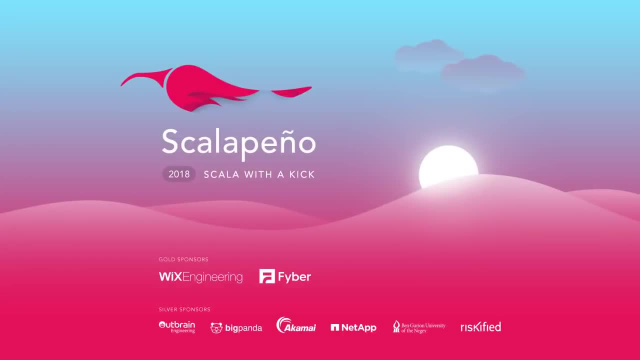 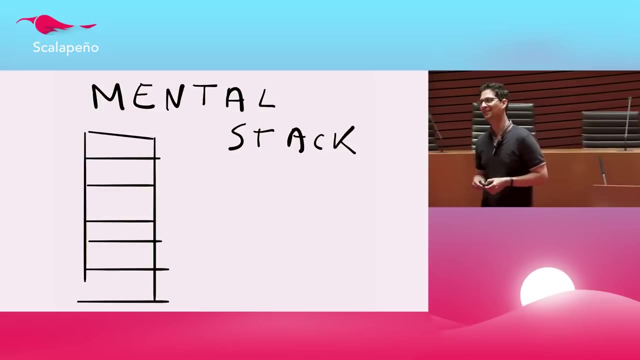 Hi, Thank you for coming. Like most of you, I used to be a Java developer. For 10 years I worked with TDD, design patterns, solid principle, and then, two years ago, I joined Big Panda and I switched to functional Scala And after a while I realized that the way 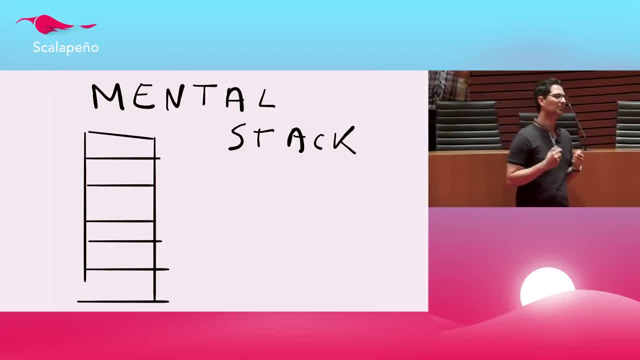 I was writing and reading code was very different. I was thinking way less, and in a good way. So my day as a Java developer would look like this: I would start with some code and in my mind I have a mental stack. 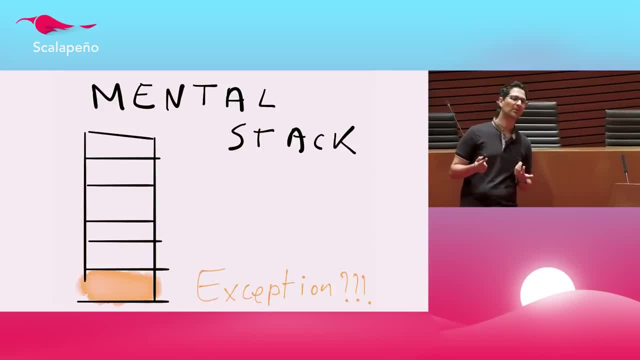 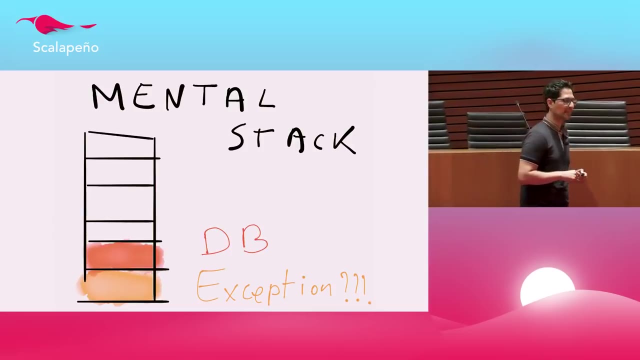 And I start to read a function and it might run exception, It might not. So the thing I have to do is to go read the implementation, see the possible exception, put it in my mental stack and go on. And then I would continue. I would read another function that would go: 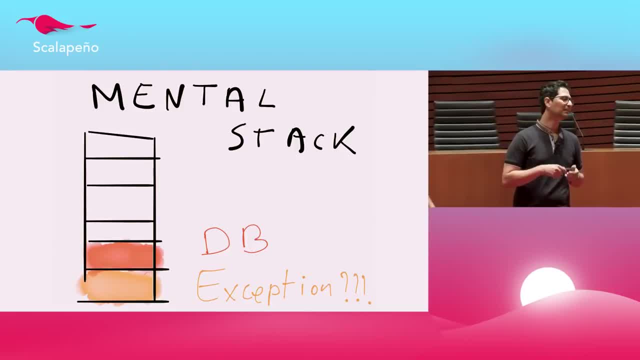 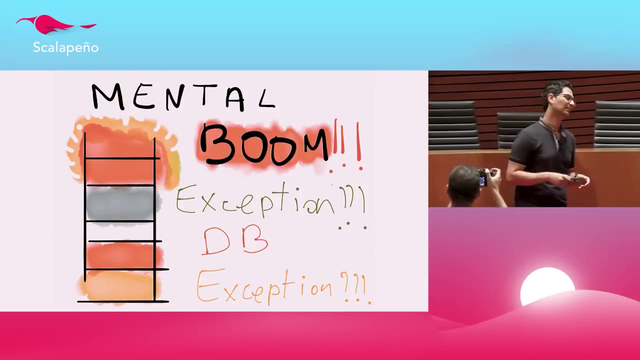 to the database And again there might be an exception, There might be other kind of errors. So I would go to the implementation, put this in the back of my mind and continue And again and again. So what happened at the end is basically overflow right, Too much stuff. 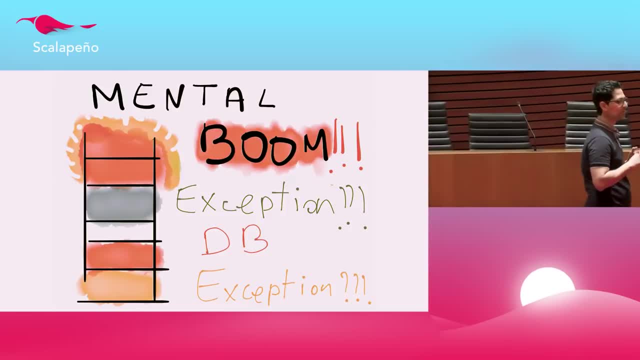 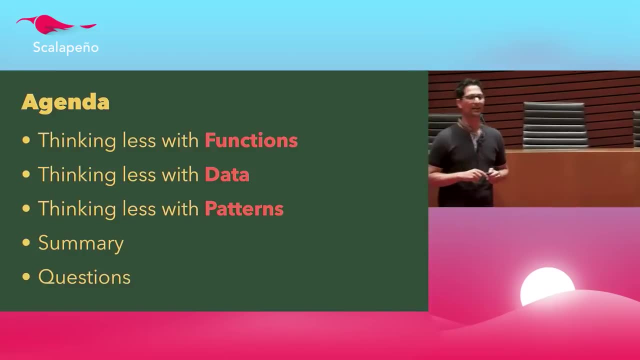 to track, and that's something you don't want to do. So I'm going to give you a few techniques to avoid that, And we're going to talk about functions. Okay, We're going to talk about data, and then about patterns, And then we'll do a quick. 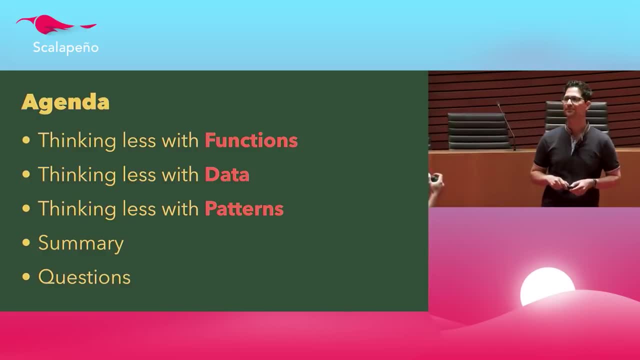 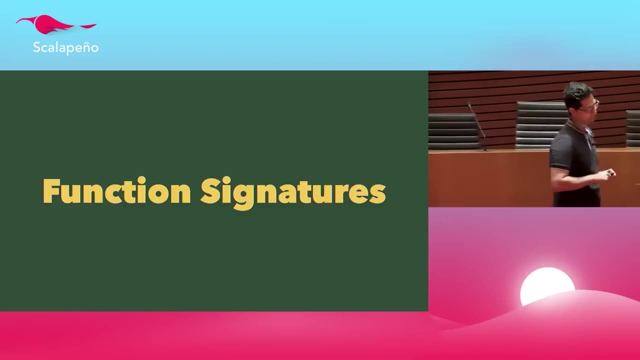 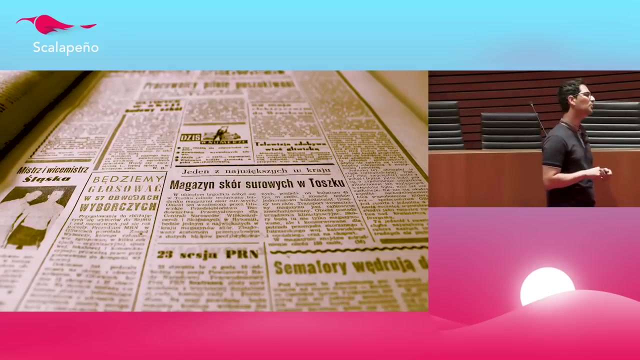 summary and we'll have questions at the end. So the first tool I'm going to talk about is function signatures. The way I think about function signatures is this way: like a newspaper. So in a newspaper you have articles and you have titles, And a good title should tell you what you want to do. It should tell you 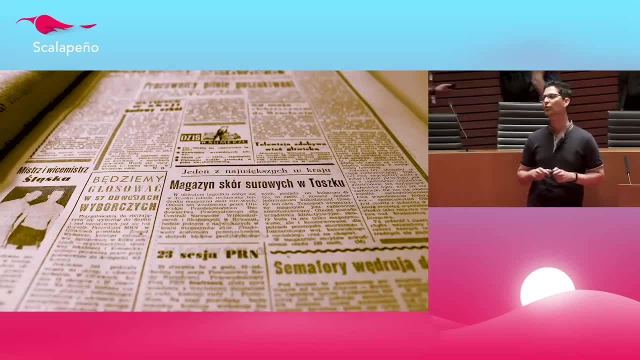 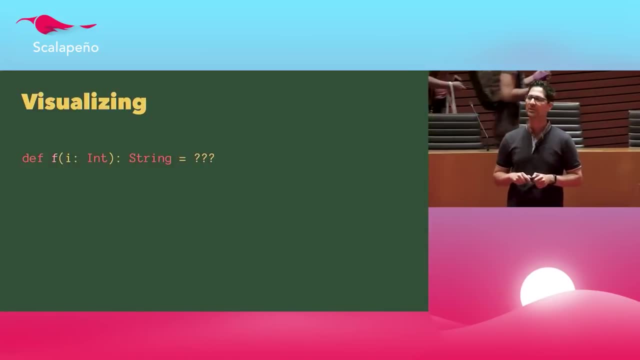 enough about the content of the article. You shouldn't have to go and read the full article. So a good function. signature should be the same way, right? So let's take a look at this function. What's going on here? Well, we have an input, It's an int And we have 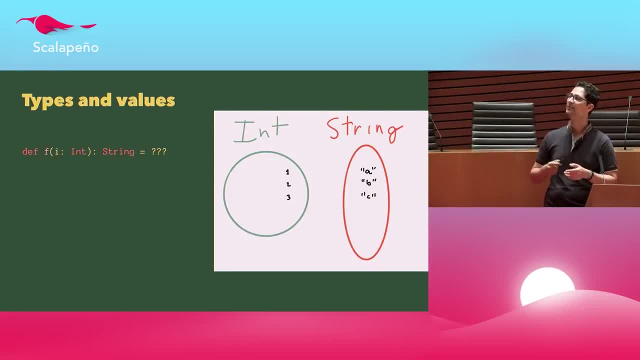 an output, It's a string. So the way to visualize this thing would be like this: We have types- Right, It's this circle Right Right ints and strings, and we have values, and values would be 1,, 2, 3 for ints, or A, B, C, whatever. 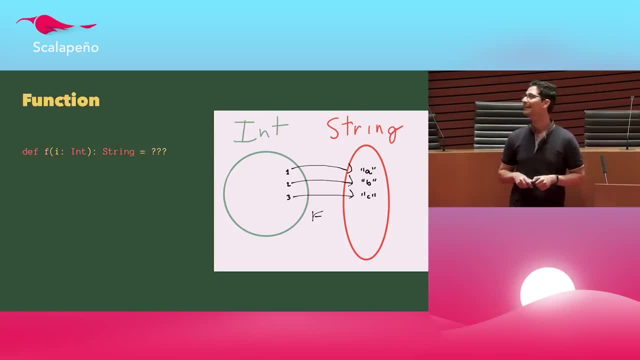 for strings, And the function is simply the mapping between those values. right, And I don't really need to know anything about the implementation. What matters here is the function signature. When I see this visual, I get the full picture right. So let's take a look. 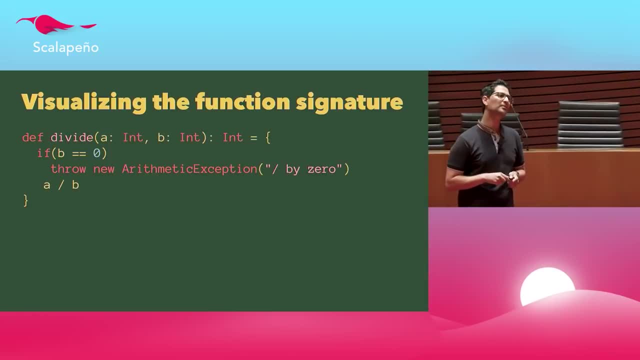 at this function. What's going on here? It's the divide function. It takes two ints and it gives me back an int. right, I'm dividing two values and I'm giving you back one, And if I give you zero, I throw an exception. So the way to visualize this thing would be: 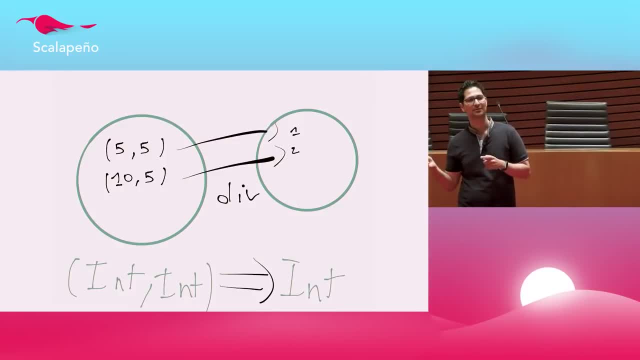 like this, right? So I give you two ints, Five and five, and you give me back one. I give you 10 and five, you give me back two, right? This visual is straightforward. But what happens if I feed it zero? What happens? 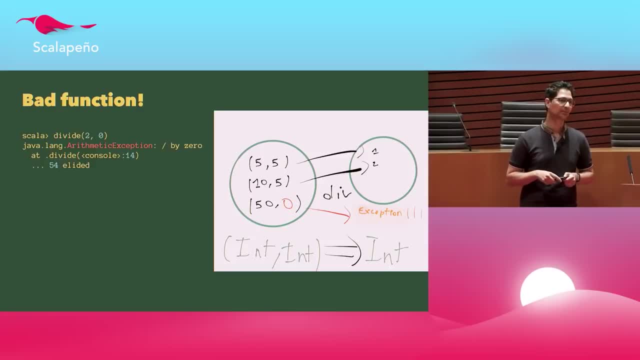 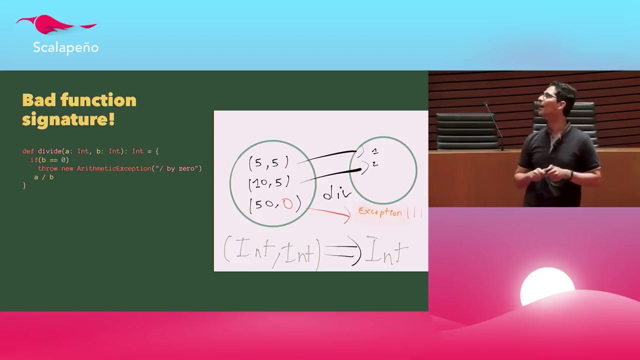 to the visual right. Well, this thing happens. There is an arrow that goes to some value that is not defined. Something not natural is going on here Behind the circle, right there exception thingy And the way right. that's a bad function signature. Why is it bad? Why? 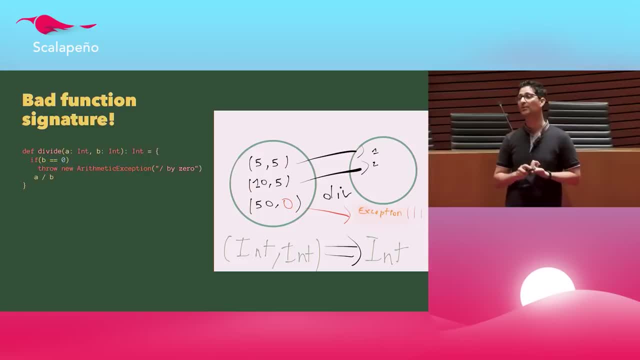 is this function signature bad? Well, it lies. It doesn't tell you the truth. You have to go and read the implementation to understand what it does And you have to keep this exception in the back of your mind. And that's only one function. Imagine a lot of those You 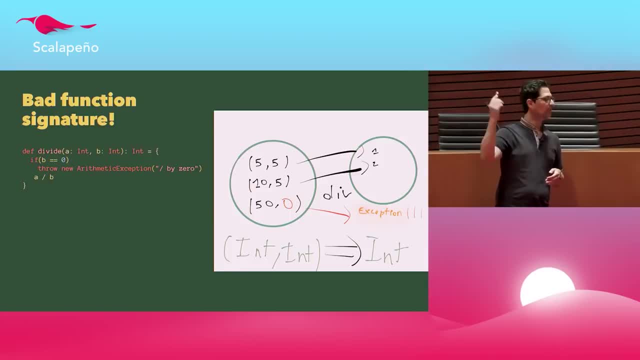 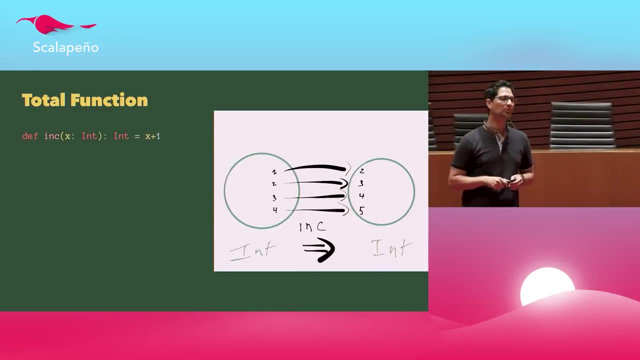 have to change those and you have to put on top of your mental stack again and again. Well, you don't want that. So the way to avoid that is to use total functions. Total functions are very simple: For every single input they have a corresponding output. So the visual 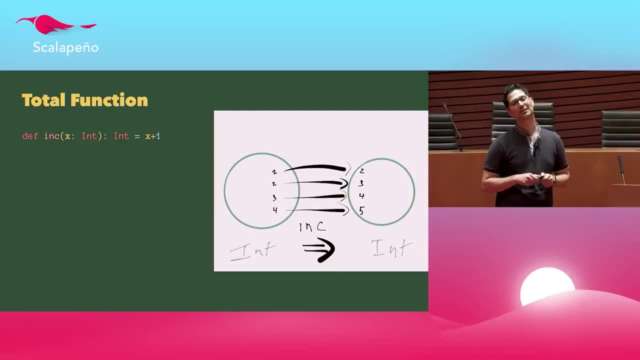 is very clean. Right. Here we have the increment function. I give you one, you give me back two. Give you two, you give me back three. It's very straightforward. The function signature is trustworthy, right? It doesn't lie to me. 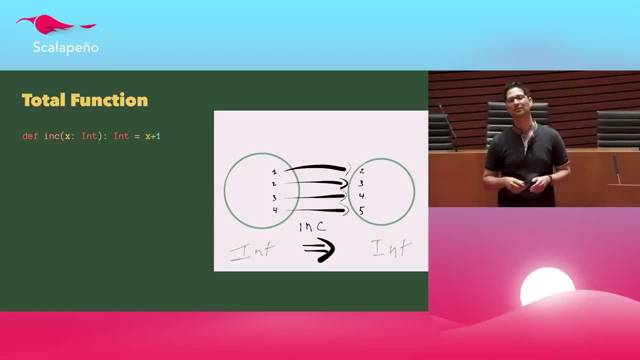 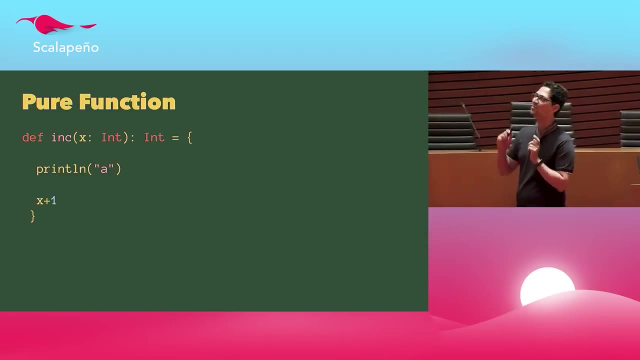 I don't care about the implementation. What I care is the signature here, and it tells me the truth. The trust is back. So let's go back now to the divide function. We'll come back to divide function after. We're just going to move to the pure function first. 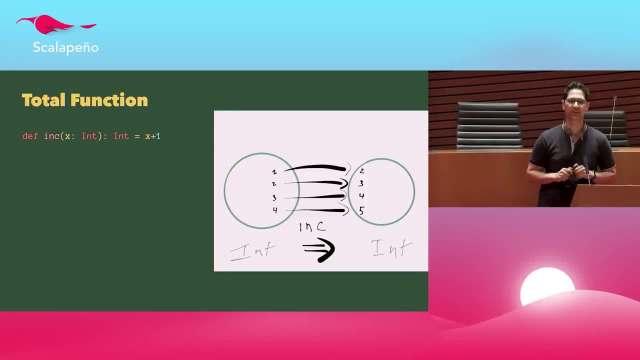 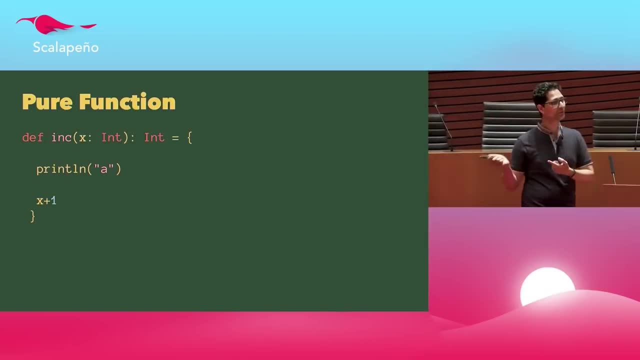 This is the same function as before, right, The ink function. here. That's the same, but something different happened here. What's different here? Is it a total function? Well, yeah, it's the same function. If I give you one, it gives me back two. 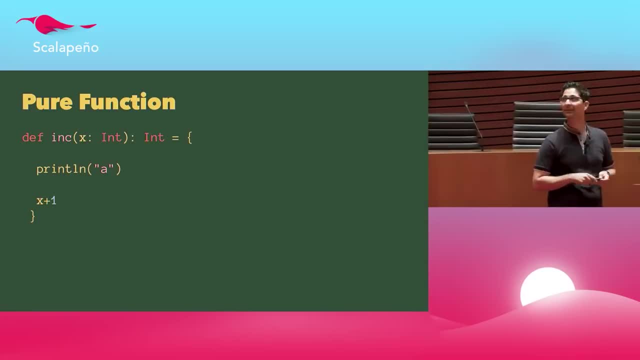 But something else going on here. There is a printing in the middle here, right, What is this? It doesn't look so bad right now, but it could be anything. Instead of printing, it could go to the database and drop the full database. 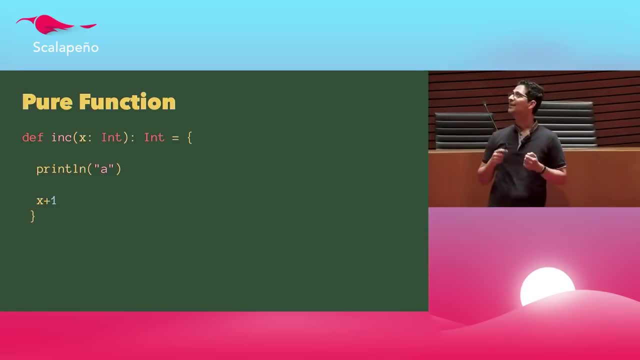 It could launch missiles. The point is, I don't know from the function signature what this function does. Again, it's lying to me. So you have to go, you have to read the function and then you have to put this in the back of your mind. 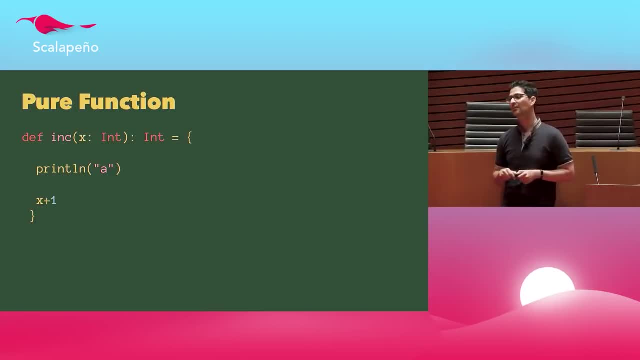 This thing is called the side effect. So you want function that are side effect free and these functions are called pure functions. right, And when you use pure function, you think less about the implementation. What matters is the function signature, not implementation. 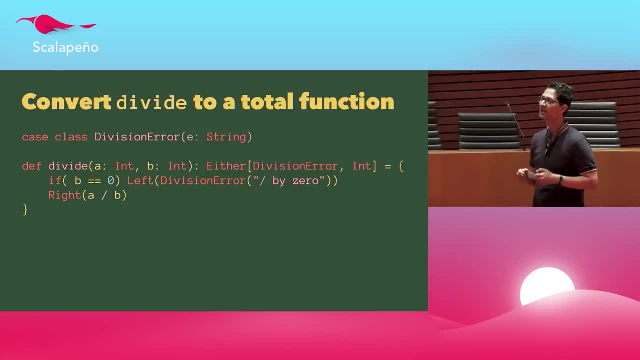 All right. So let's go back to this divide function and let's try to fix it. So the way to do it right is to use this container type, called either: And it will tell the reader of the function that there might be an error. 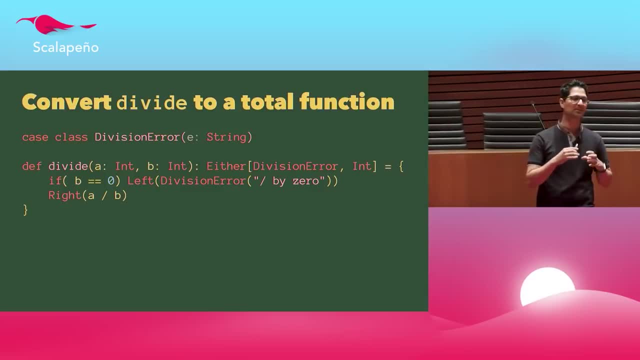 in the function right What it's doing. basically, it's bubbling up the internal of the function at the level of the function signature. This either type would tell you: on the left side, that's the errors right And on the right side, the good value. 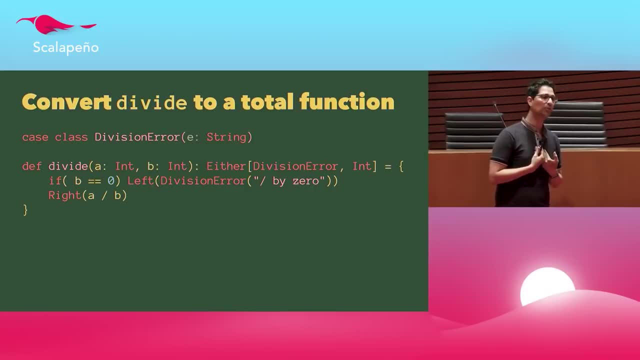 So now, as a reader, I don't have to go and read the implementation. I can just look at the function signature and that's it. I get the full picture here. Right, We're going to talk about these container types now. 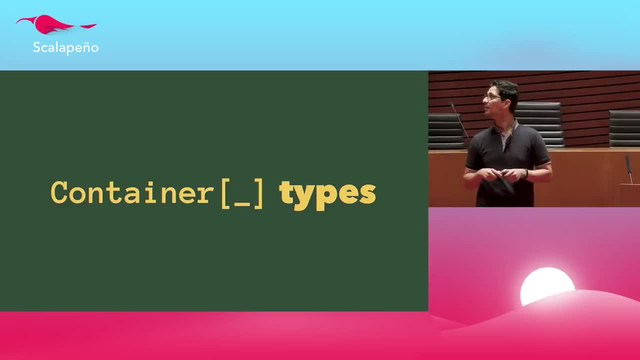 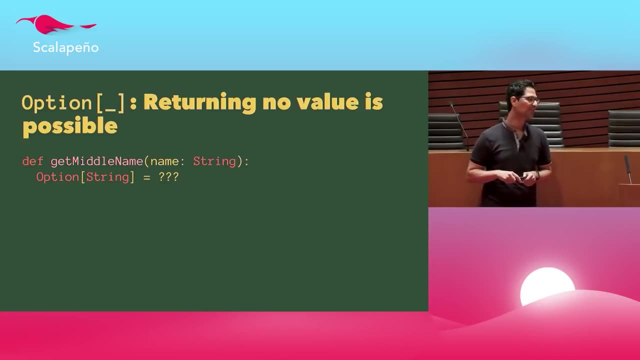 We're going to review the most common ones quickly right In the standard library in Scala. So one of the most common one is option. So I would have a function like that which is middle name. Not everybody has a middle name. 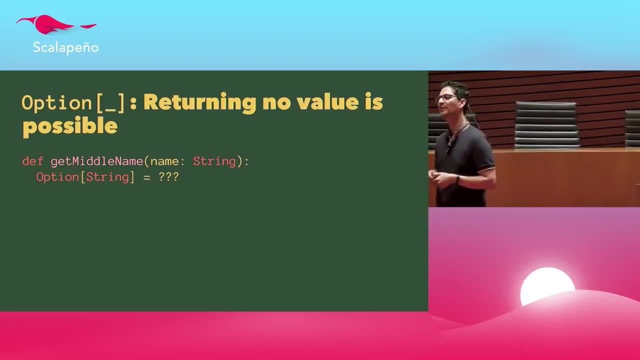 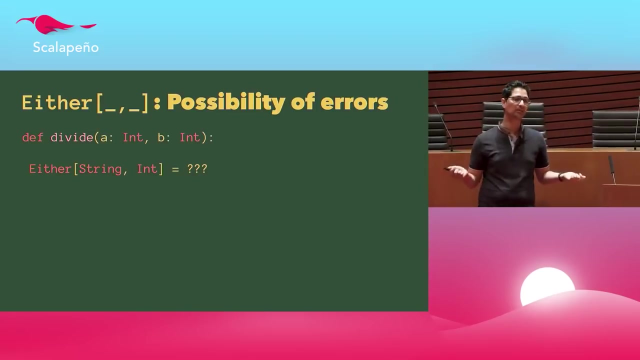 And when I read this function signature, it will tell me there might be a return value or there might not. right, It's all about readability and to express yourself to the reader of this function, Either we just saw it now. So when you have a function that retains an either type right, 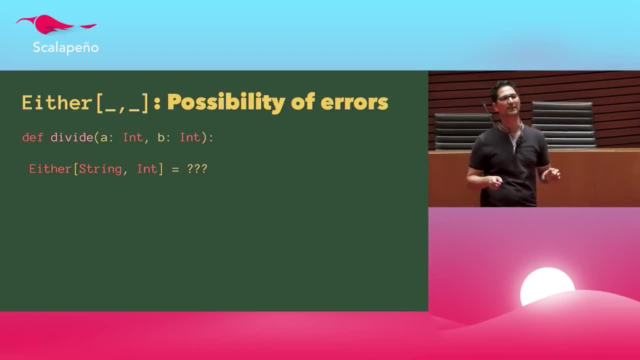 Basically this container type. just wrap the simple type right. That's what we do here. You see, there is this bracketing thingy. So inside you put the type that you would like to return And here again it will tell you: this function might return errors. 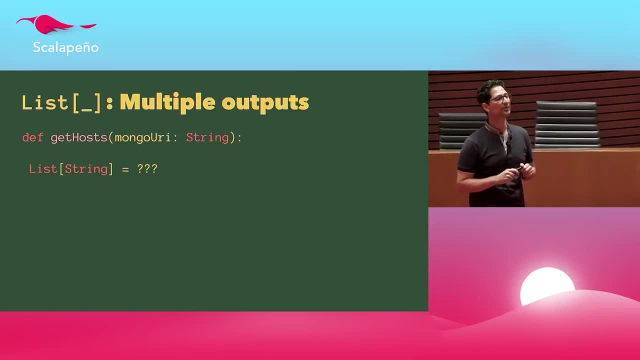 Right, We have a list, and this is a little bit different. It's talking more about the shape of the output. When you read this function right, it will tell you you might have multiple output values. It's a little bit different than before. 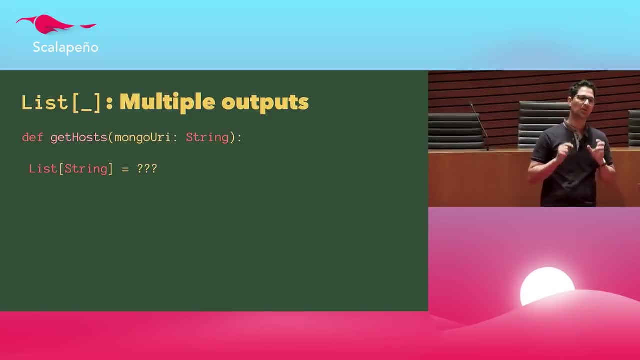 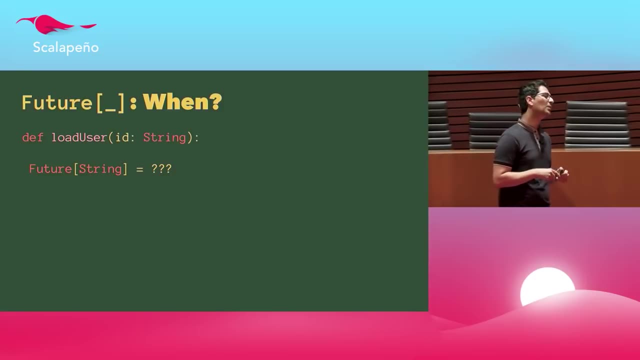 We don't talk about errors. We talk about the shape of the output values. Then we have future. That's also very interesting. Future will tell the reader of the function that the value that is expecting might be or might not be available right now. 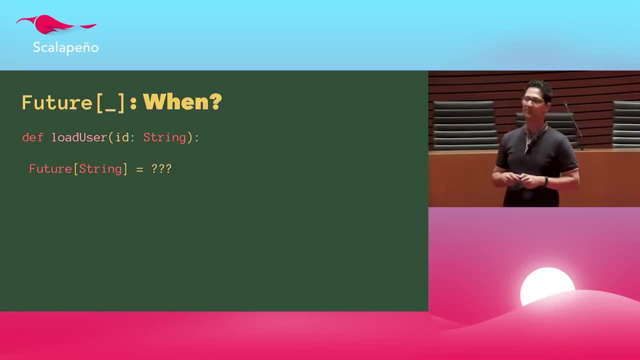 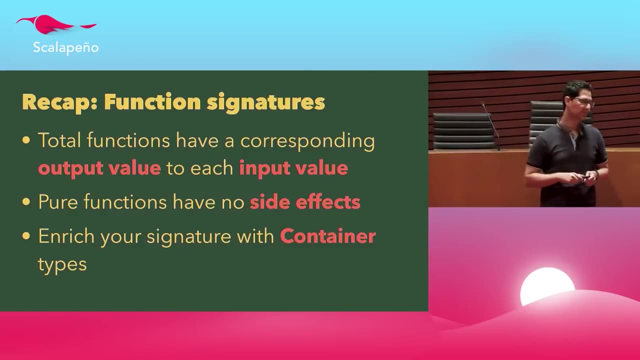 It's more about when this value is available. All right, So let's recap quickly. We talked about total functions, And now for every input, you have a corresponding output. We talked about pure functions that have no side effect, And then we talked about container types, right? 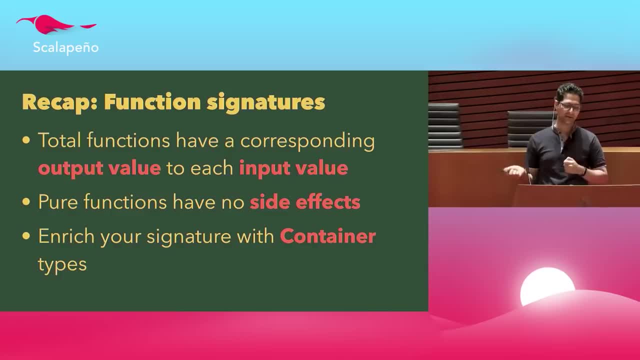 We saw how we fixed this divide. function with either and you have to. when you use all these techniques right, you get, you enrich your signature right. You give a new meaning to your signature. Think about the newspaper, right. 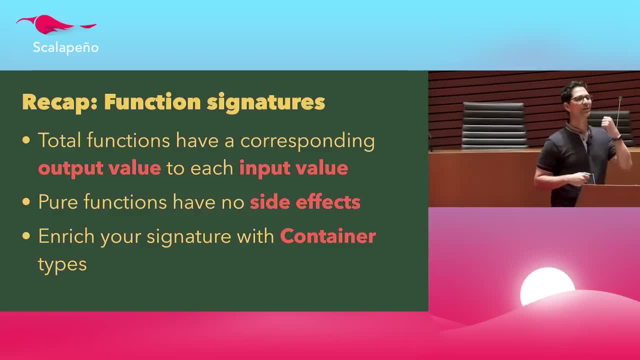 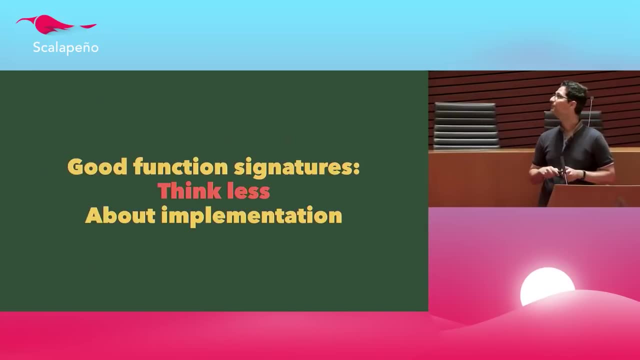 You want a good title. You don't want the reader to go and read the full article, You just want to give him a good headline. So good function. signatures make you think less about the implementation. That's the whole point, right The mental stack thing. 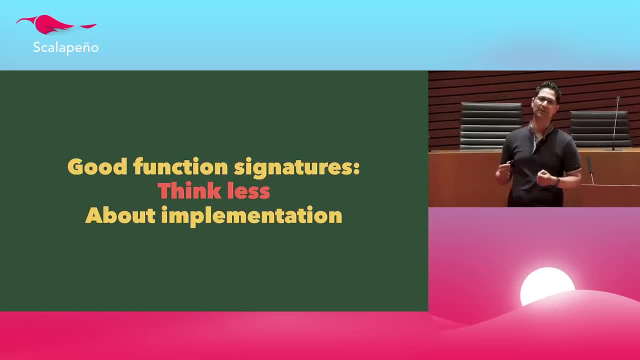 You don't want to go and read the implementation every time. That's what I used to do in Java. always, I would just click on the function. Everybody is doing this. Look, look it up. What is it doing? You don't want to do that. 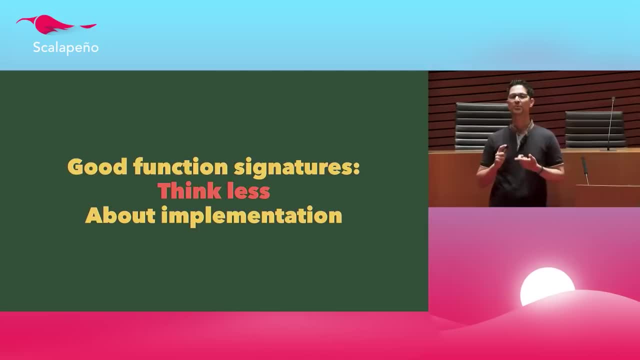 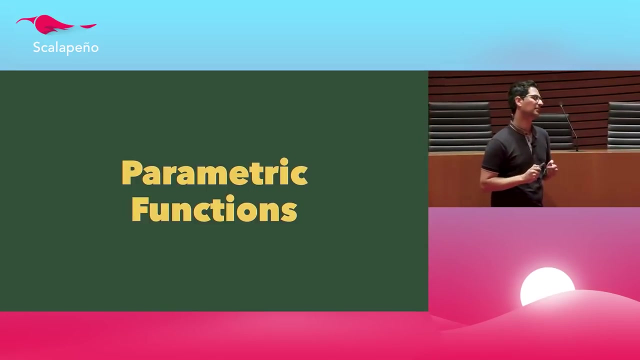 You don't have to do that. When you use total functions, when you use pure functions, when you use container types, you have good signatures and you don't have to think about implementation. All right, Now we're going to talk about another property of functions. 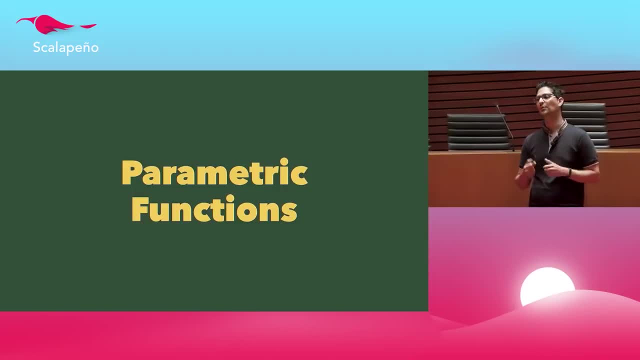 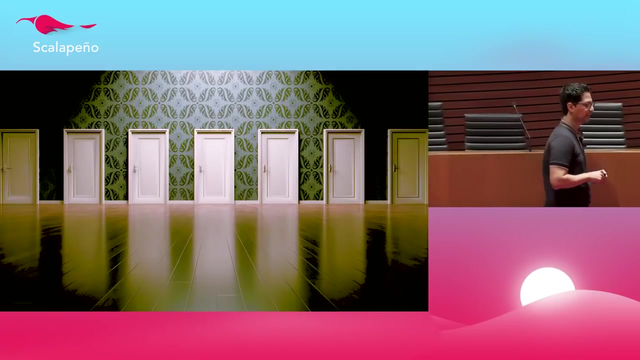 And it's a little bit different. This was a big aha moment for me. in functional programming. It's not so much about if I care about the implementation, but more about how many ways could you implement the functions. It's very interesting. 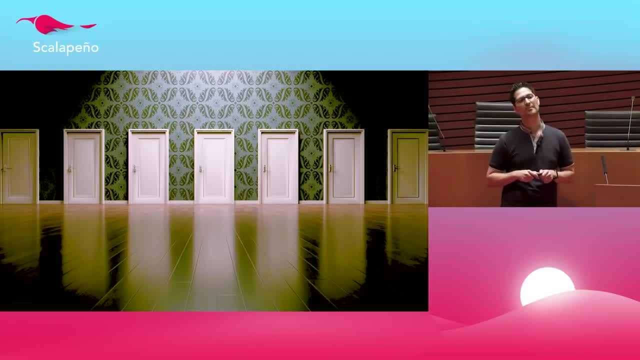 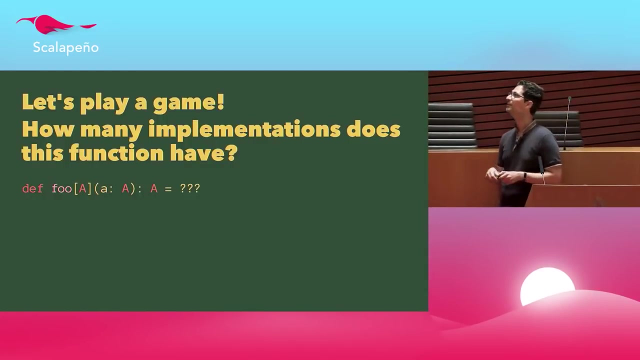 Think about writing a function. You have a function signature and I give you a pen right, And it could be 10 pens. You don't know how to write this function. There are so many possibilities. So let's take a look at this function, right. 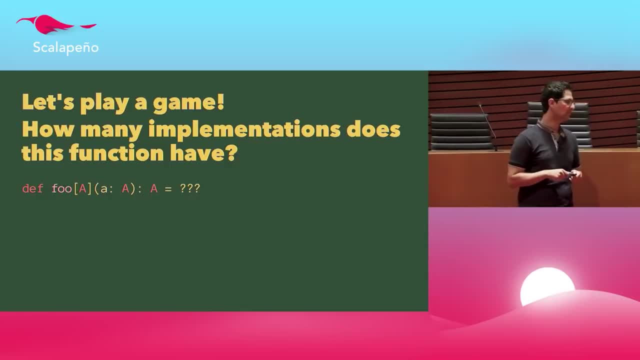 And this is a parametric function. So we have here a parametric type a. This thing tells you in the bracket what it tells you: that you could replace this a with any type: Could be a string, could be a long, an int, a list, whatever. 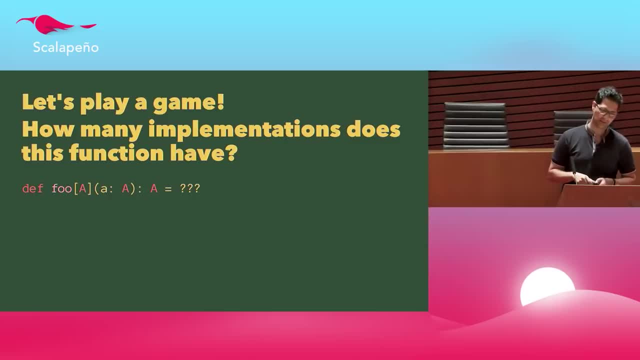 That's what you have to think when you see this parametric type. And the question is: how many ways could you implement this thing, Could you implement this function? Of course we're using total functions, pure functions. We don't use side effects. 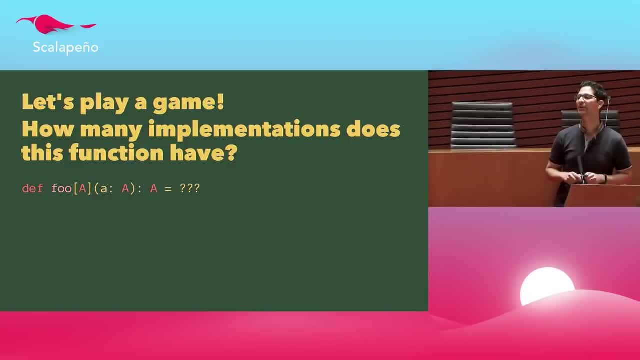 We don't throw exceptions And we're restricting ourselves not to use all this magic hash code functions, Right, Yeah, Yeah, Yeah, Yeah Yeah. Two-string functions, all the stuff that comes from the object Java class, right? So how many ways? 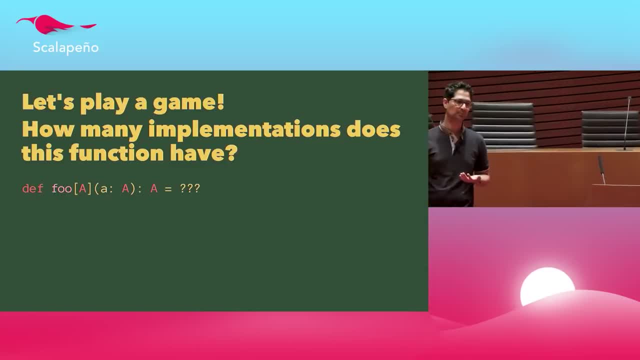 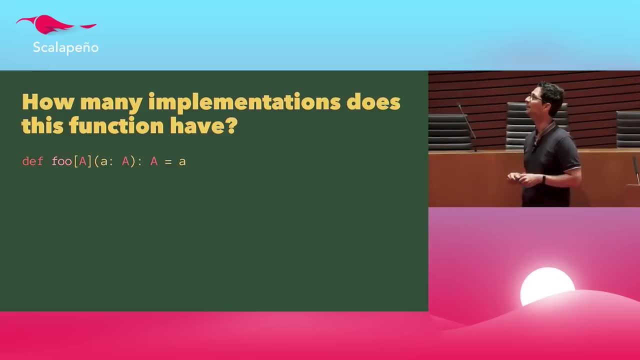 Two, three, four. Well, it turns out there is only one way to do it Right, And what's interesting here is: why is that? Why is there only one way to implement this function? So the answer is easy. 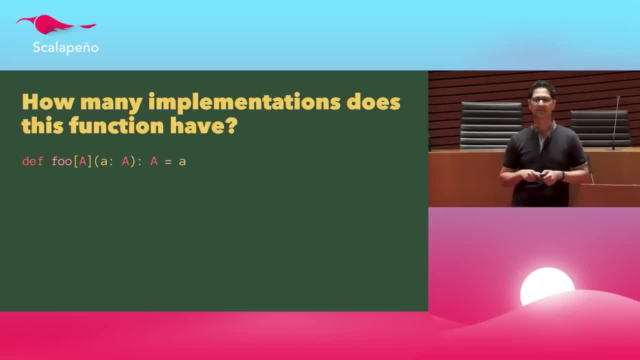 We don't know anything. anything about a. This thing is so abstract that I don't know its values. If I tell you int, you can draw the circle of ints in your mind and you know the value: one, two, three, four. 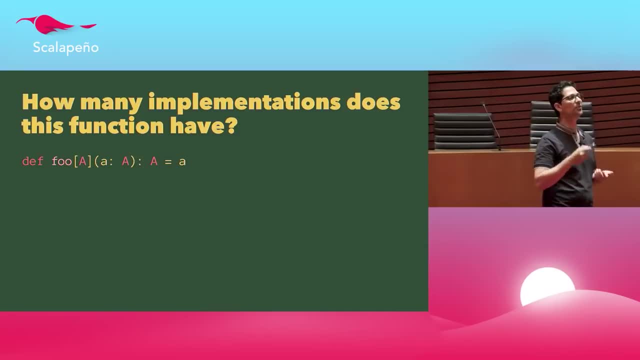 But if I tell you a, you draw this circle. You don't know its values, You don't know any function on a, So you put into a corner here. you have no choice. You have to return the input. You have only one way to implement that. 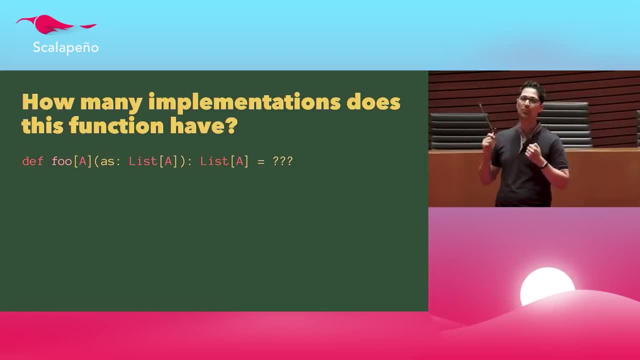 What if I do that? What if I enrich the type signature with a container type with list? I'm doing a small thing here. I'm just changing this a into a list of a and I'm returning a list of a. So what I'm telling to the reader? 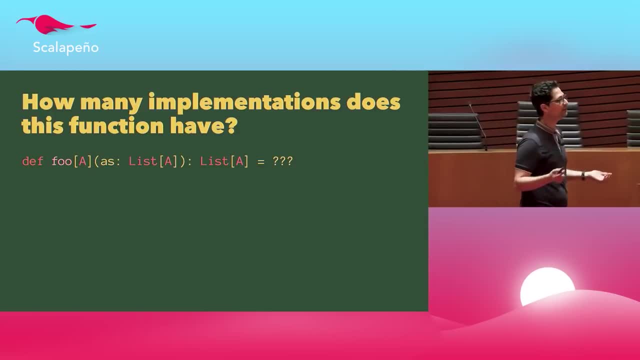 is the shape of the input could be multiple a's and the output could be multiple a's. How is it going to affect the number of implementation? How many ways could you implement this function now? What did it do to the implementation space? 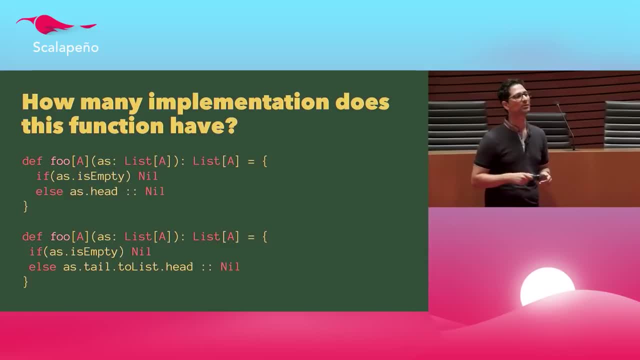 Well, we can implement it a little bit more. We have a little bit more possibilities. We can switch the head and the tail. We can do some stuff, but not so many. We can't sort this thing. We don't have any ordering on a's. 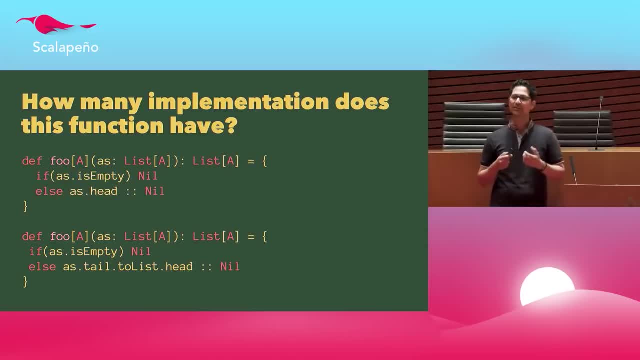 We can't sort the list. So what happened here? basically, We just enriched the function signature with a container type and we get a little bit more of implementation space. The way for you to write this function is a little bit more. There is a little bit more ways for you to do it. 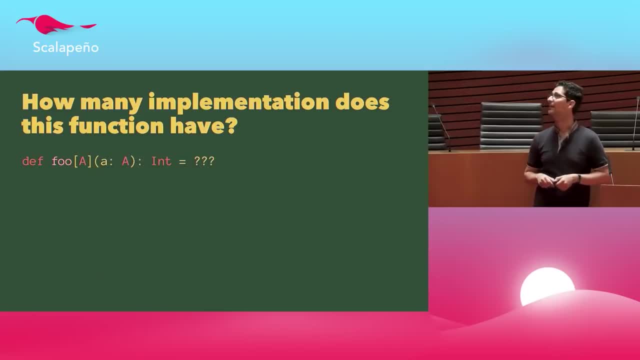 And the last one would be to do something like that. What would this do to the implementation space of the function? What did I do here? I just removed the a as a return value and put an int right. And think about it again. 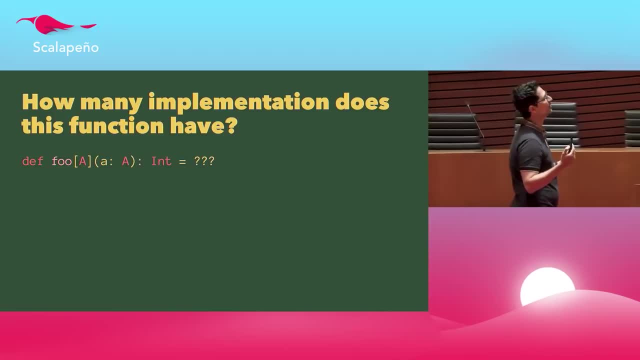 This int. you can draw it in your mind. It's a circle with the values 1,, 2,, 3, 4.. So how many ways can you implement this? Well, 1 can return 1,, 2,, 3,, 4,, 5, the number of ints right. 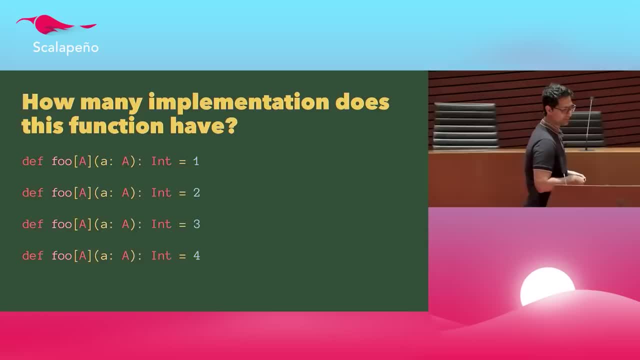 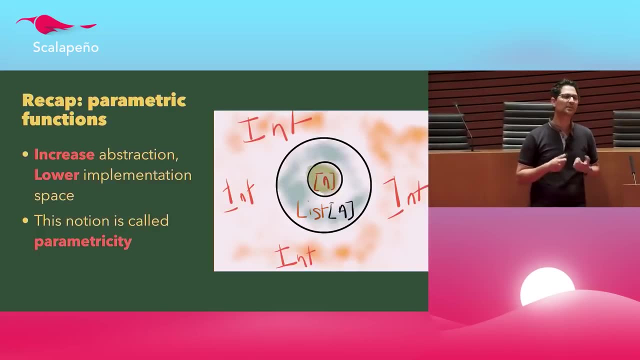 So what happened here? What happened? Let's think about that. We just jumped here. Let's look at the dimension of number of implementation. That's interesting. We started with something very abstract, with 1a right, And we had only one way to implement it. 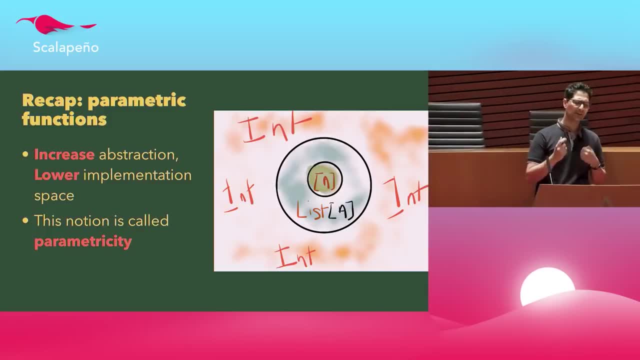 And then we enriched the signature with a list. We had a little bit more implementation possibilities, but not so much, not so much. And we finished with int and we just jumped to another dimension. So what does it mean, this thing? 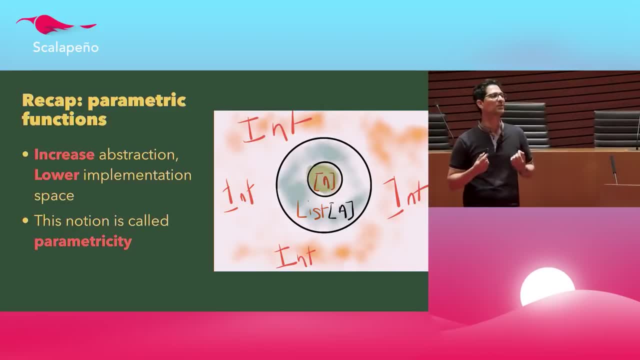 Well, This notion is called parametricity And it's very interesting. Why is it important to you? Because when you use a parametric function, right, the more it's abstract, the less way you have to implement it, the less possibilities for you to make a mistake, right. 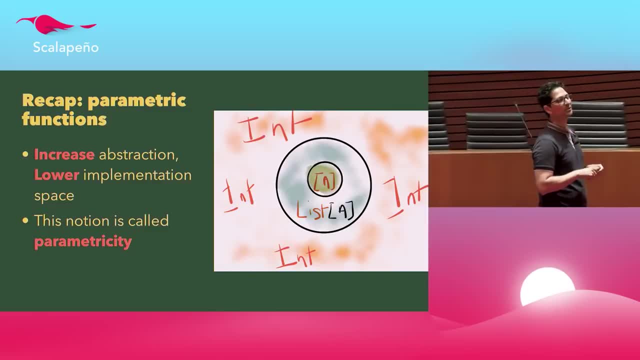 It's like giving you a blank page and I give you 1 pen, or if I give you 10 pens, So you have so many choices that you could make mistakes. But here, when you use parametricity, the more abstract it is, the less you. 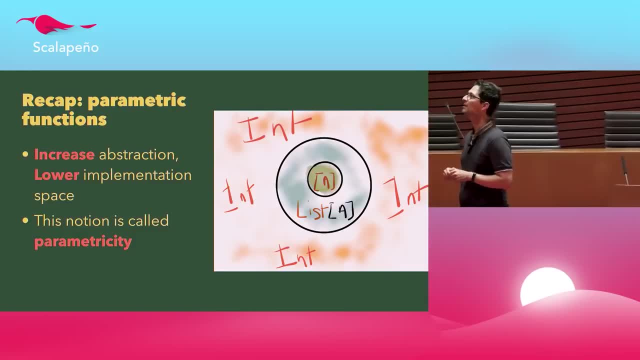 have to think about how to implement the function right. It's not so much about what implementation is with the function signatures. It's more about for you as a developer, how to write the code right. You have to think less about it. 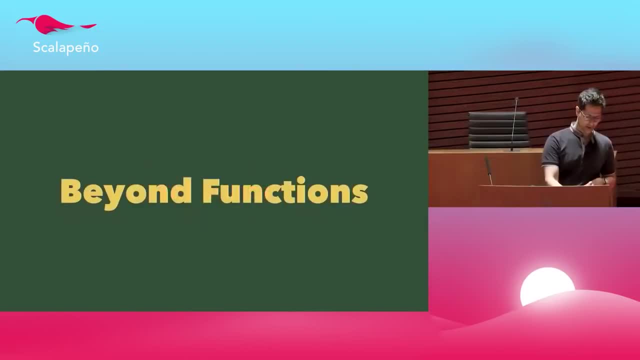 Makes you think less about your implementation. So we talked about functions right, About total functions, Functions, pure functions, parametric functions. But of course functional programming is programming with functions. But we all know that software is not only functions right. 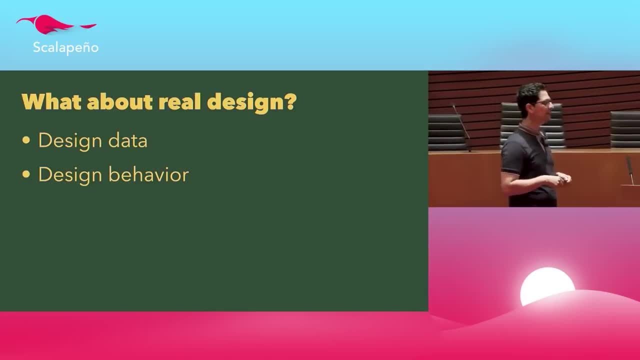 Function, like software, is about designing data and designing behavior. It's beyond functions. right? There is something else there. If you want to build a full-fledged application, you can't just start writing functions. It's not going to work out. 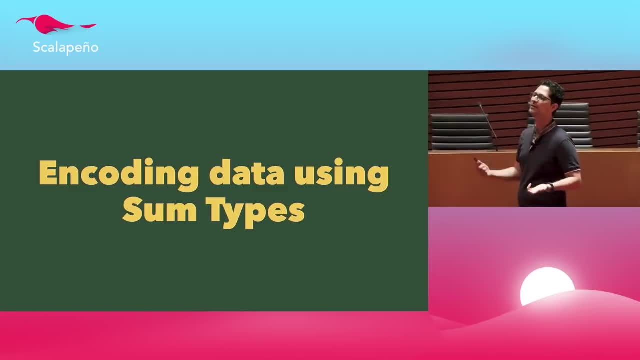 And is there a way We're going to start with data? So is there a way to encode data that would make you think less, that would have this property for you, as a developer, to think less, in a good sense, right? 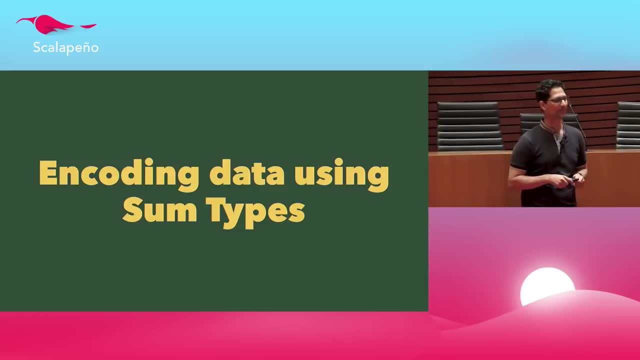 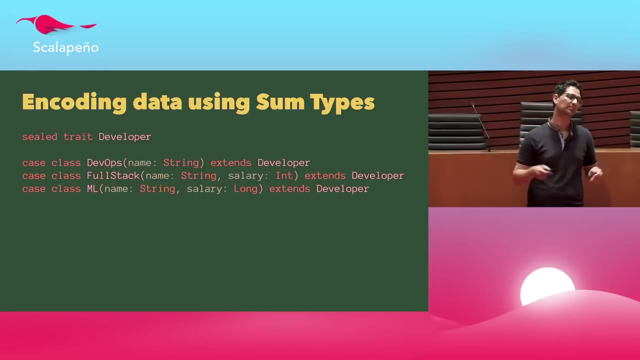 So the way to do it is to use sum types. Sum types is a way to encode data, So it's very simple. Here we have a developer trait which is basically an interface, And you would have a DevOps which extends this developer trait. 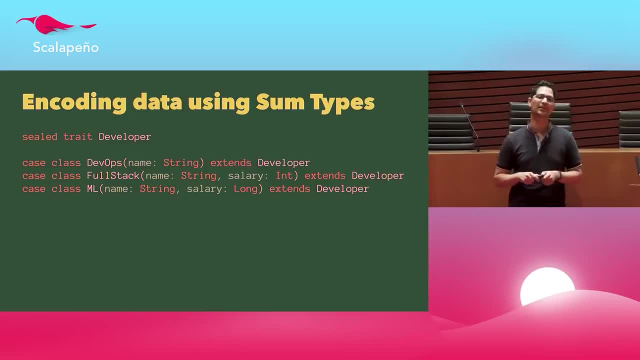 Then you would have a full stacker with a salary in it, And then you would have an ML developer with a salary in long. And what does it really mean? this thing right. Why would you want to encode your data this way? 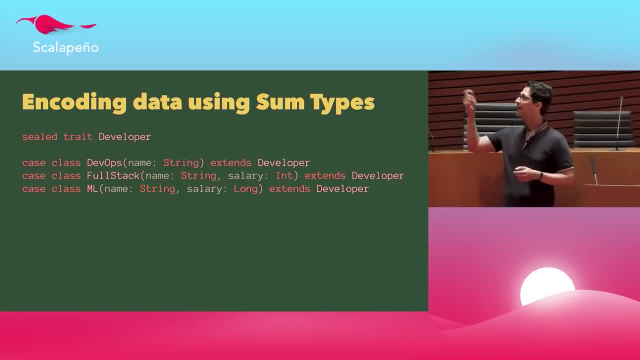 Why would you want to use this sum type pattern? This, The pattern, sum types- is also referred as algebraic data types, So keep this in mind. And why would you want to do that? Why would you want to use that? Why is it a good thing? 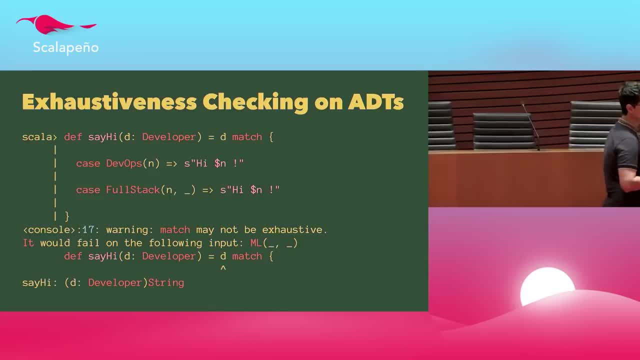 Well, first, the compiler will be with you When you use this thing. if I write a function, say hi, that takes a developer and I pattern match on it. if I forget a case, the compiler will tell you: you forgot the ML case, right. 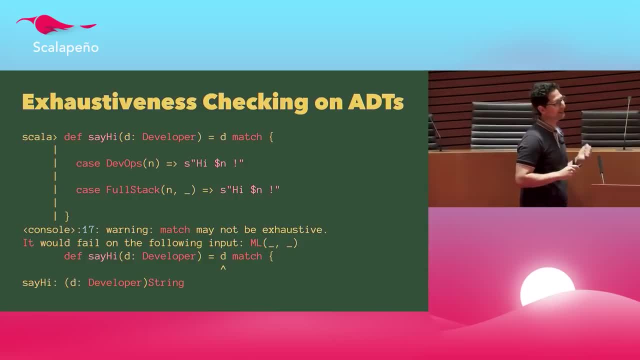 Something that is extremely powerful. In Java, the compiler will only check the syntax if you forget a semicolon or like a bracket. Well, in Scala, it will check the correctness for you. something that is very powerful. A lot of functional programmers will tell you. 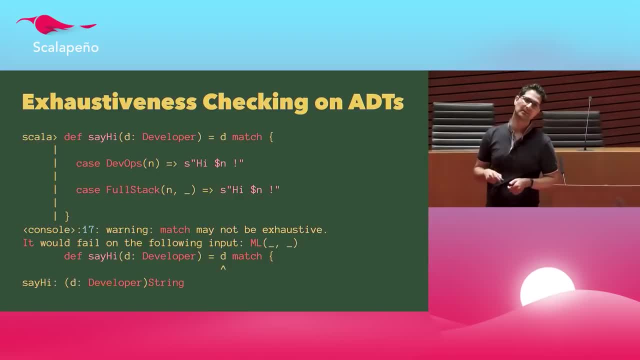 you know, if it compiles, it works. Well, it comes from that, Because the compiler, The compiler is not only checking the syntax, but checking the correctness of your code. That's why they would say that Also, these ADTs, these sum types, well, they're immutable. 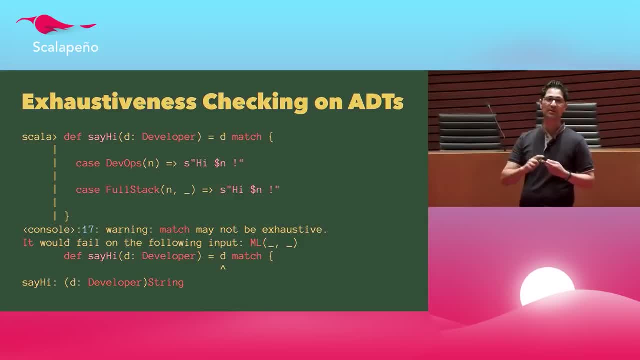 So you don't have to think so much about concurrency bugs, shared mutable states. You can't change this stuff right, This developer? you can't really change this. If you want a new instance of it, you have to create a new one. 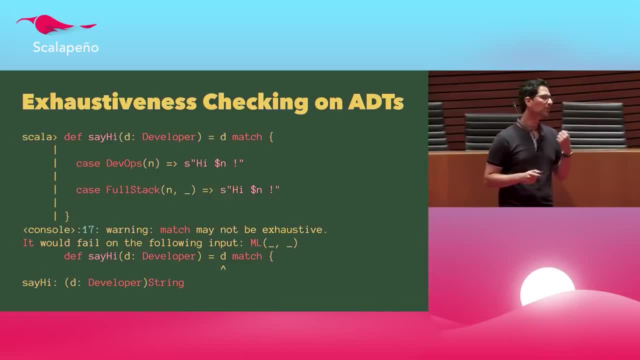 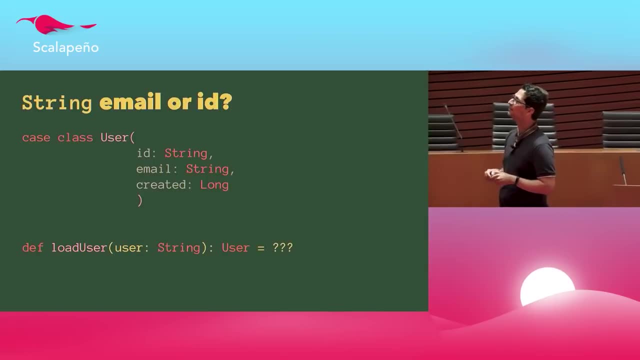 So you don't have to think about all this possible mutable shared state. All right, So what about this function, the load user function? Well, you've seen it in a lot of code bases. You know these strings everywhere, these ints. 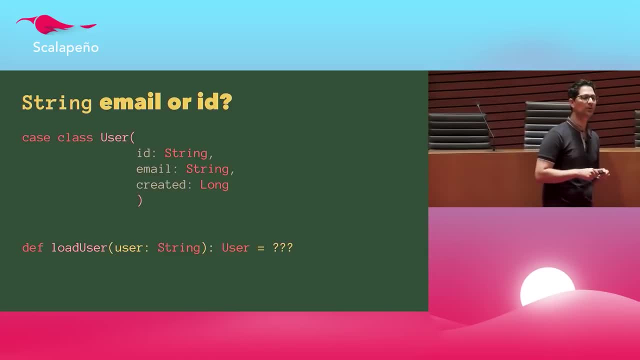 these slungs. You don't really know what it is Right here. this load user could use the ID, could use the email You don't know. You want to encode your data to make you think less about all these possibilities. You want the compiler to work for you. 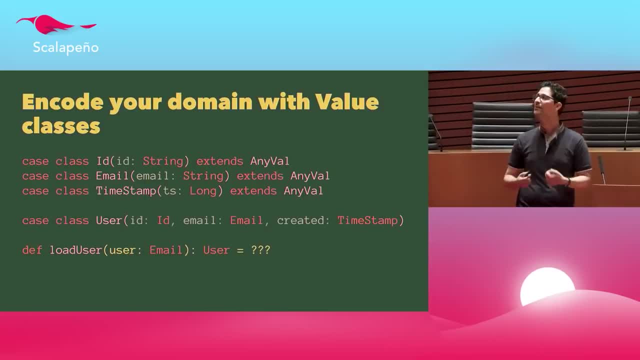 And the way to put some domain knowledge in your values right. I want this load user function to take an email, So the way to do it is to use value classes And basically these value classes. it's just a simple pattern. 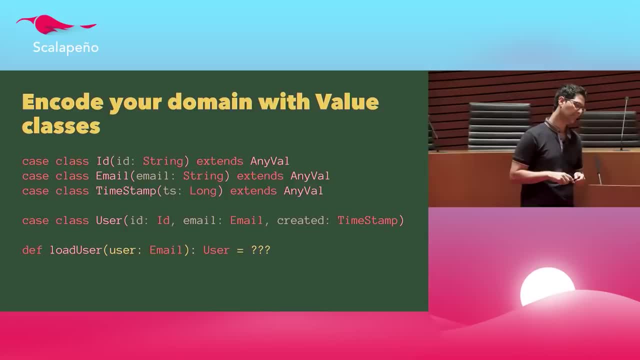 You wrap your simple type and you extend any value And now you get a nice type. right. My load user takes an email. What does it do really? Why is this thing important? Because you're putting domain knowledge inside your types. 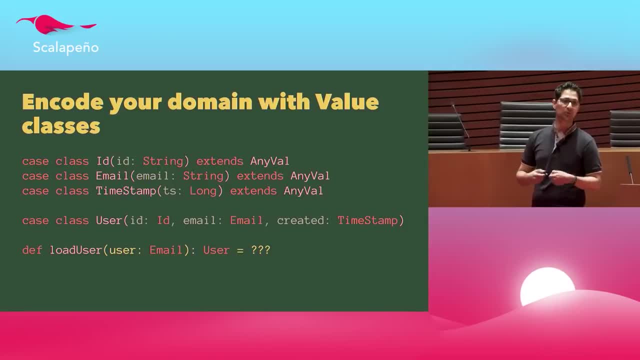 The compiler now will be behind you to catch you when you make a mistake. You don't have to think so much about what these strings longs, what they mean. these doubles, Is it money, Is it time? No one knows right. 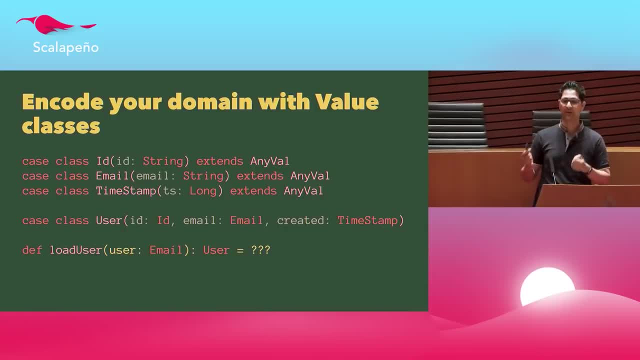 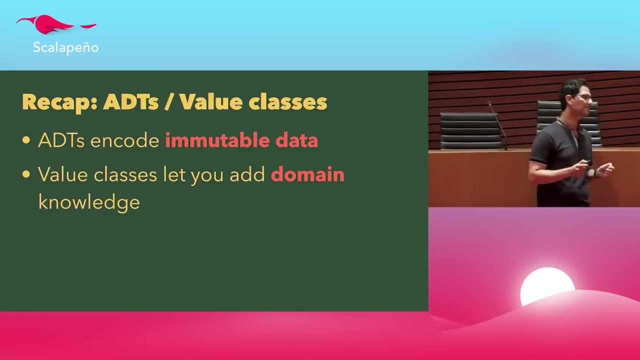 But if you type it properly with value classes, you don't have to think about that. All right, let's recap. We talked about ADTs, right, about some types and how they encode immutable data and how the compiler will check the correctness of your code. 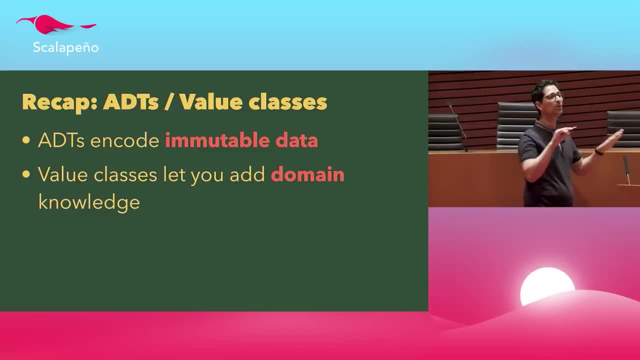 when you forget an edge case. Basically, there is no more edge cases. You don't have to think about forgetting a case. The compiler will do it for you. We talked about value classes And how we can just put domain knowledge inside the types. 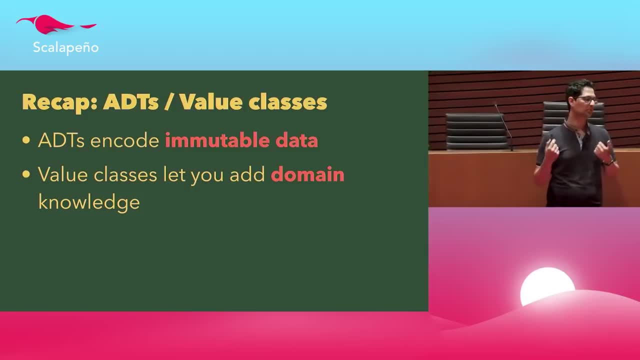 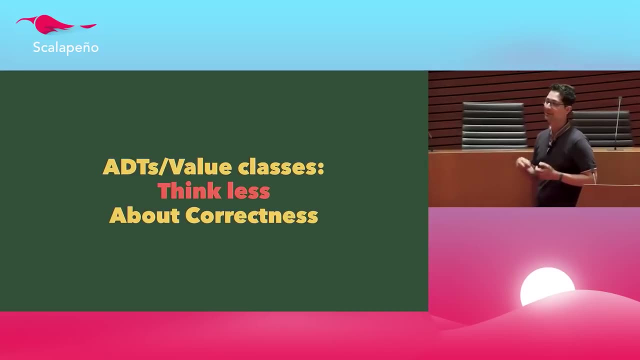 so the compiler will also help us to write code that is more correct. So all these techniques right about data will make you think less about the correctness. You don't have to think so much like before. The compiler will check the correctness for you. 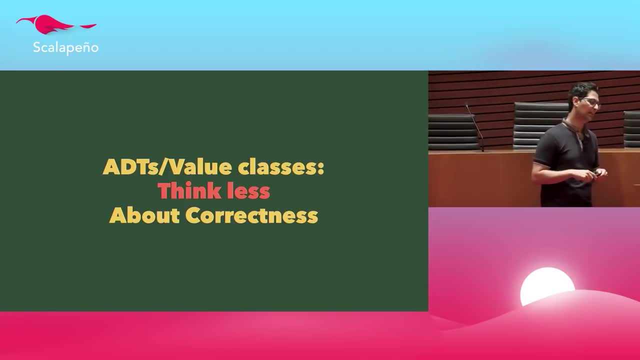 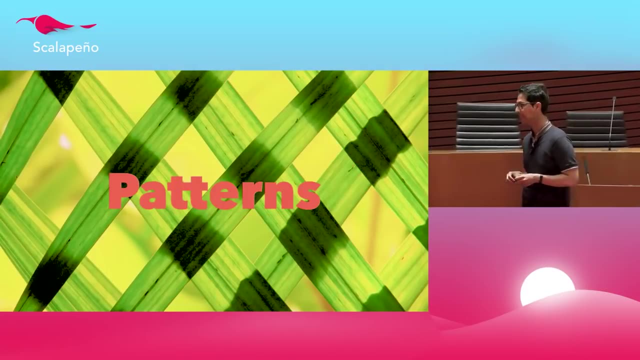 something that I believe is extremely powerful, And Java doesn't give you right, All right. So we talked about functions, We talked about data And what's left? Well, patterns, right, The way to design software in the old world. 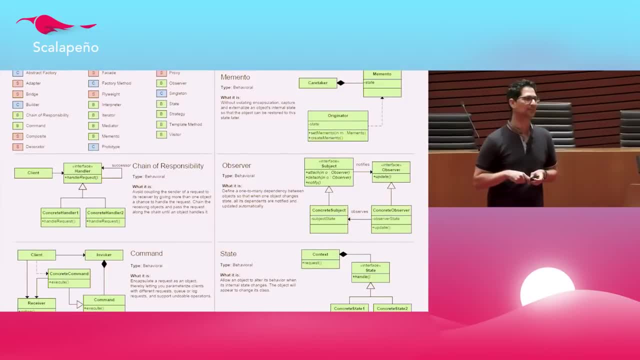 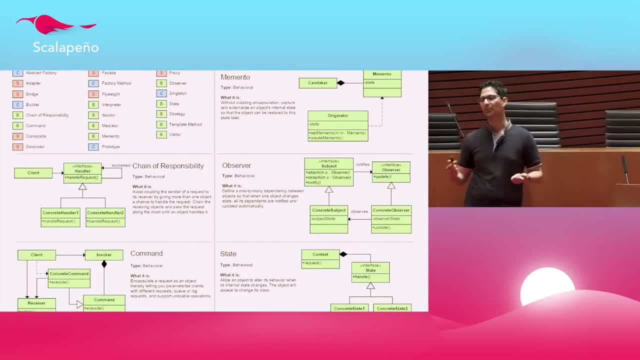 All these patterns do emerge in your software. You do see them. You do see abstract factories, visitors and stuff like that, But they sit in a book somewhere. right, Every team that you work- I'm sure you've seen it- will implement these patterns. 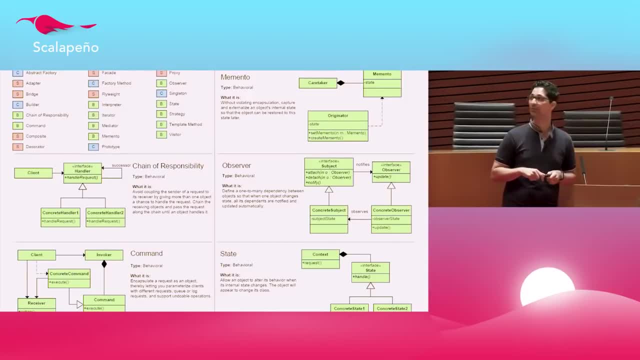 in a different way. Also, when you start learning those- it might have happened to me- you start using them everywhere. So what you get is all these over-engineered code bases. It takes a long time to internalize these patterns, So is there a way right to fit this in your mental stack? 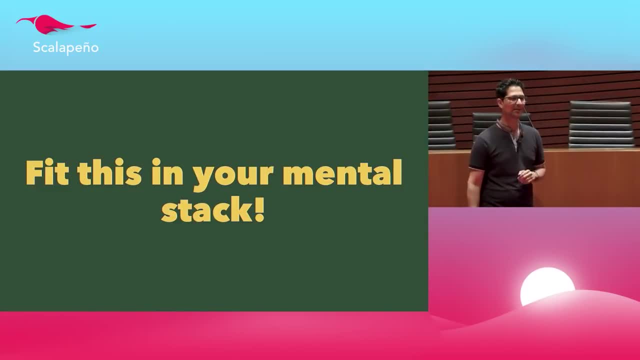 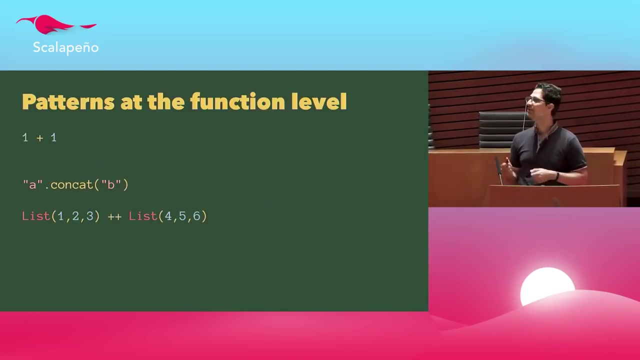 all these patterns? It is not. It's not that easy, right? So is there a way to design patterns, to have patterns that would make you think less, right? You won't have to fit all this stuff in your mind, So let's go back to the function world. 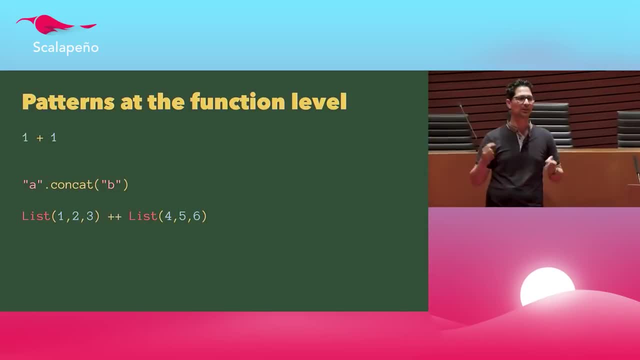 and try to do patterns at the functional level. OK, So how would you spot patterns The old way? Well, you would look at your code, you would refactor and then you would see a lot of similarities. So here it's the same thing. 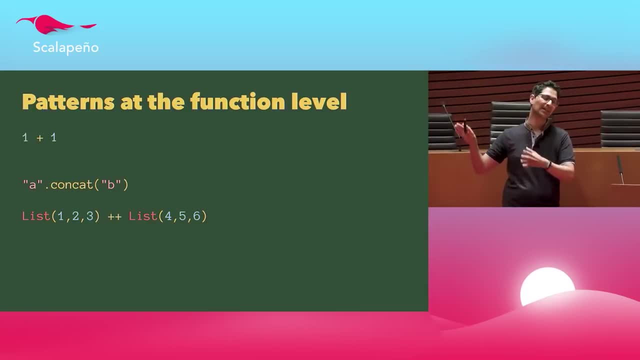 It's exactly the same thing. You have to look at your functions and try to spot the similarities right. And what are the similarities at the function level? Well, the number of parameters, the number of outputs, the type right If the types are the same- the shape of the functions. 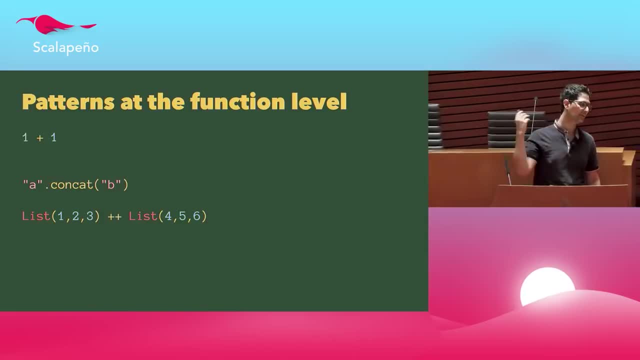 So here I have 1 plus 1, A concat B, List 1,, 2, 3 that I want to concat with list 4, 5, 6.. So what does all of this stuff has in common? 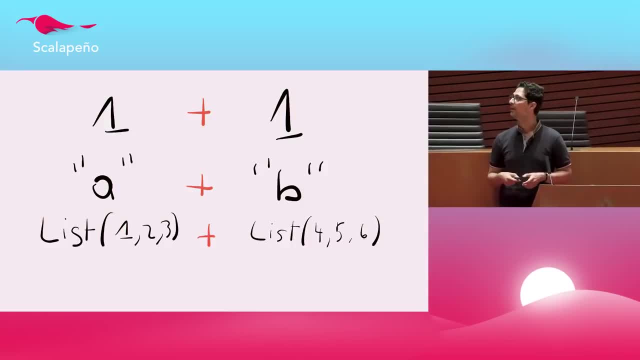 Let's try to find a pattern here. Well, they have the same number of parameters, right? I give you two ints, you give me back one. I give you two strings, you give me back one, right, So they have the same number of parameters. 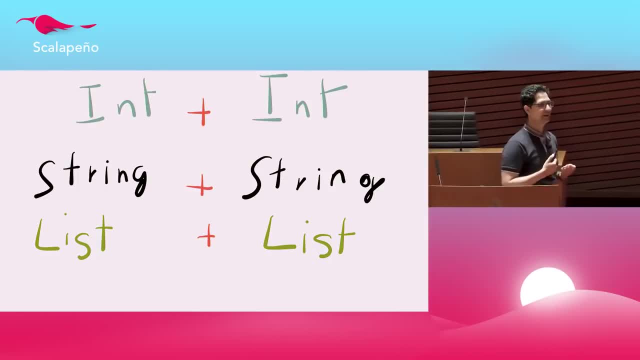 Also the type. It's the same. right, I give you int and int. you give me back an int. That's the type of similarities you have to pay attention. now, right, It's very different from design patterns. Now, you don't look at classes and hierarchies. 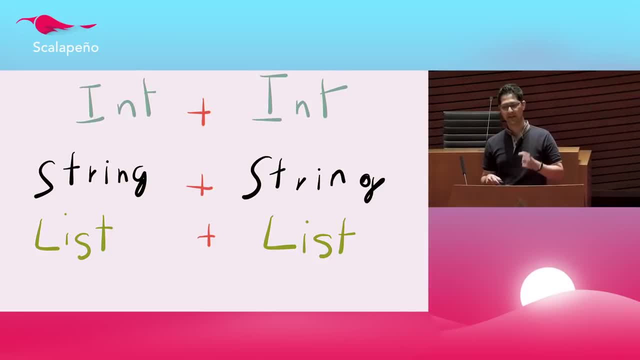 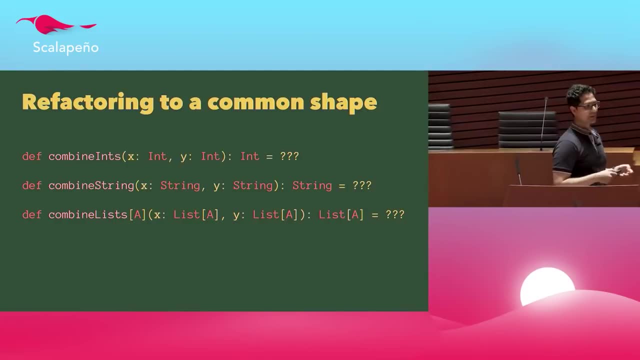 You just look at your functions, at your types, at your parameters and you try to see similarities. So this stuff, you would refactor it to this type of function, right? Combine ints. I give you two ints, you give me back one. 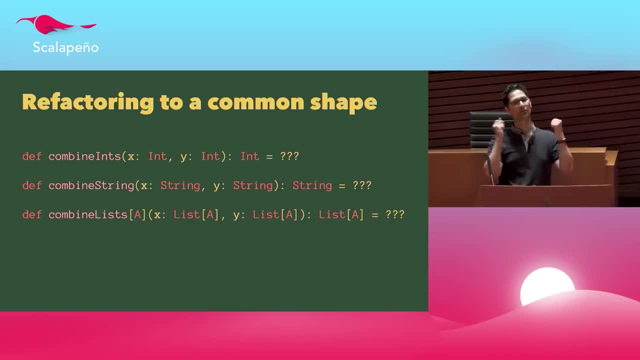 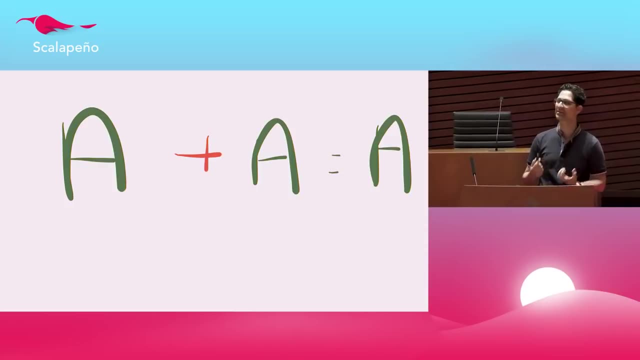 Combine strings the same. I give you two of strings. you give me back a string. Same thing with list. And what is the essence of this stuff, right? What transpires out of this pattern? How can you capture that? Well, it's this thing, right. 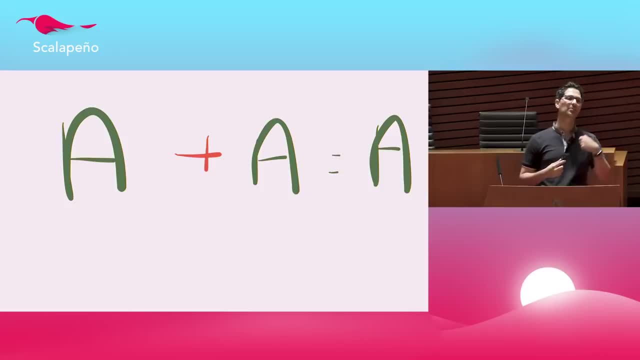 You can feel it. It's one A and another A and I give you back an A. It's one type, two of the same types, and I give you back one. And how would you encode this thing in code? How would you do that? 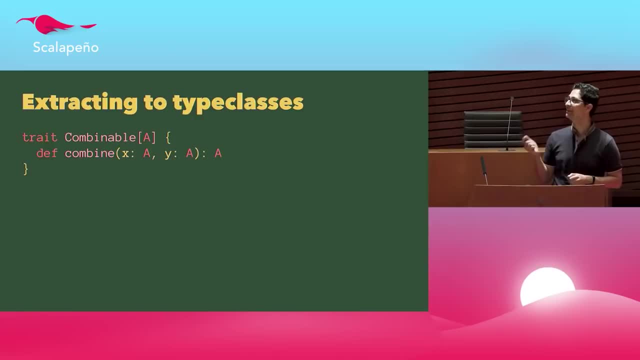 Well, the way to encode this is to use type classes. That's the way to extract the similarities at the function level. And type classes are not classes, They are traits. right, It's an interface. They have type parameter. We see here A And the function that we wanted to extract here. 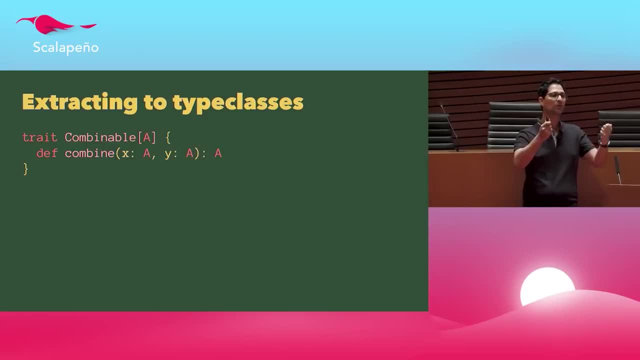 this combined thing is here. It takes two A's and gives you back an A. It's very abstract, We don't have an implementation, But we can feel that this is the right encoding And this is a parametric function. That's the tool for the job, right? 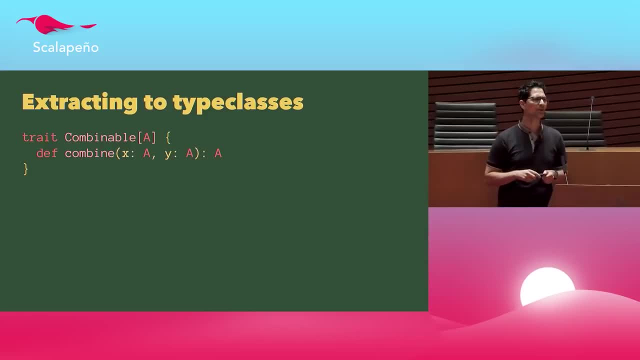 A parametric function. It's very abstract, right? So, all right, now I have this stuff. What do I do with it? right? What do I do with this? How do I use this thing? right, It's so abstract. 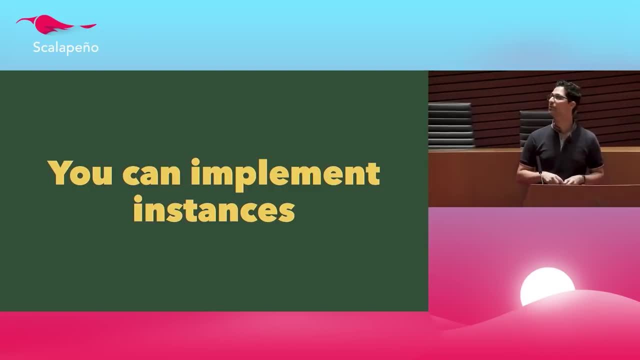 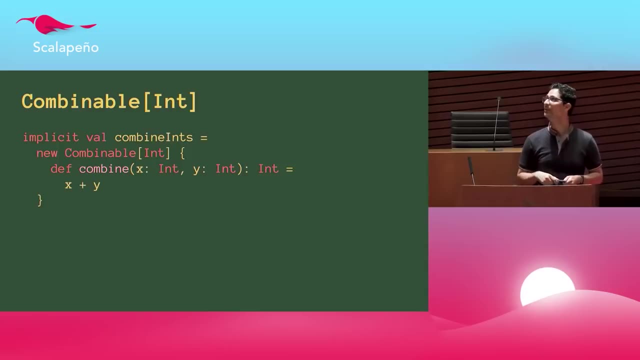 Well, One way to do it. One way to do it would be to implement instances. So it's very tedious. right, It's manual, You just do a new And you override this. combine with your own type. So here we do, for int and int. 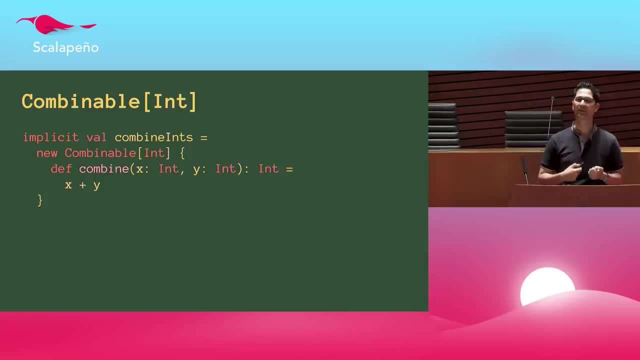 And we supply the implementation for combining to int. Here we decided to do a plus. Same thing for strings, right? I override this. combine method with string and string And I give you back My implementation of it. You can also do it for your own types, right? 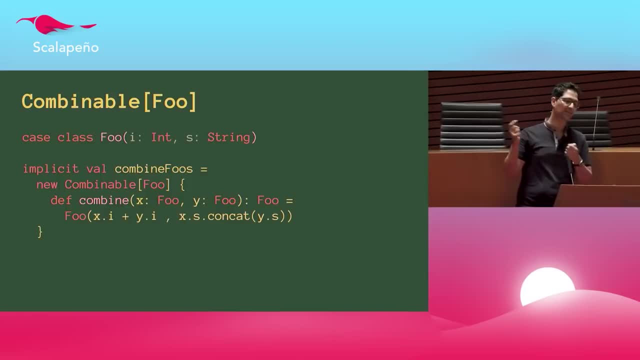 Here. I created my own class foo, And it takes an int and a string, So I can also implement the combine method for foo. right, It's my own implementation And I tell you how to do it, So I would take the first parameter and the second one. 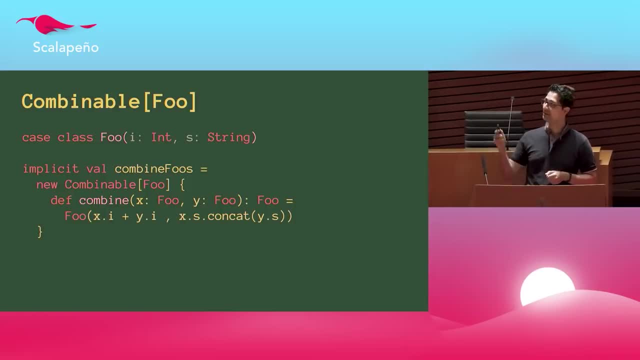 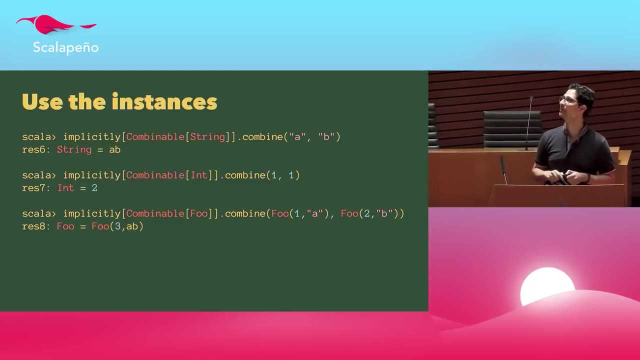 And we give you back a new foo, This stuff also, you can pay attention using places. That's the way to do it. So why we use implicit? Because we want to summon the stuff and get it magically with the implicitly syntax right. 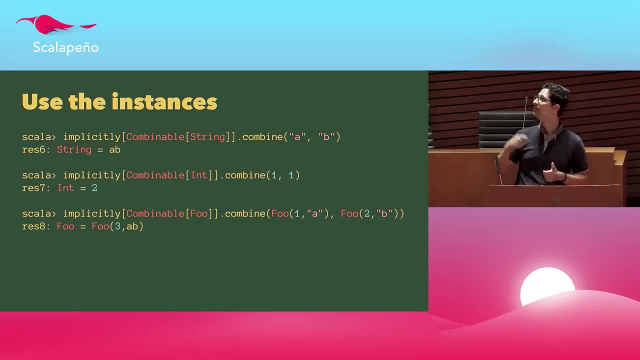 It's very nice. You see, I give a and b, I get a, b, 1 and 1, I get 2.. And same thing for foo. Great, OK, That's a nice refactoring. It's very nice. 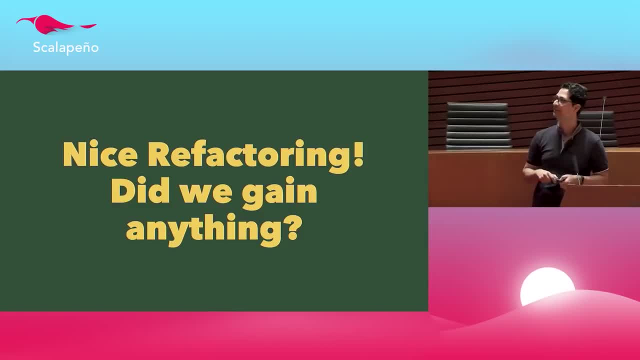 But did we really gain anything here? Did we gain? Did we gain something right from the old way? Well, first of all, we don't use class hierarchies, right? All this scary XML stuff just doesn't exist anymore, right. 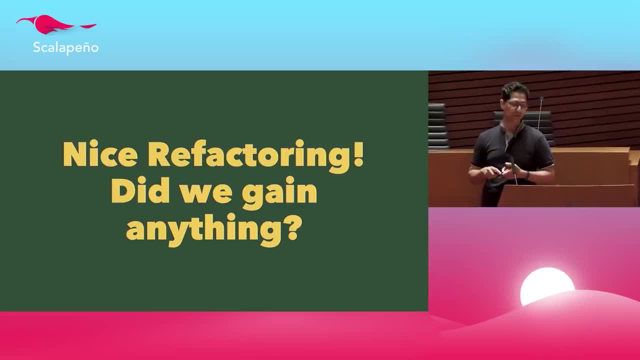 We work at the function level right. So we didn't use any inheritance here, right, We just use overloading. We didn't use inheritance. And, like design pattern, this stuff has a name right, One of the strongest aspects of design pattern. 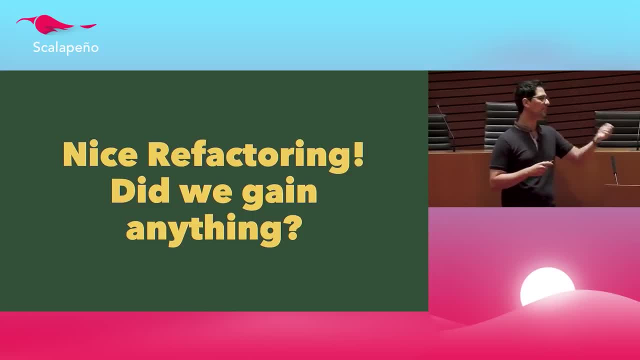 is, they have a name. So if I'm in a team and I tell my coworker I used an abstract factory, it's supposed to know what it is. So the same thing with these functions, with this pattern. These patterns have a name. 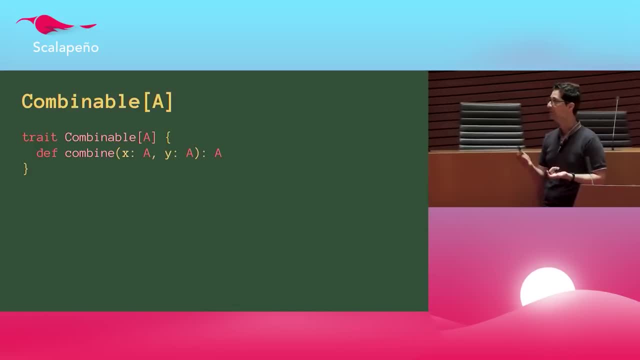 And this combinable thing that we just discovered. its official name is a monoid right. So this stuff right all this, and that's not the only thing. There is a lot of these patterns And a monoid. it's the same thing. 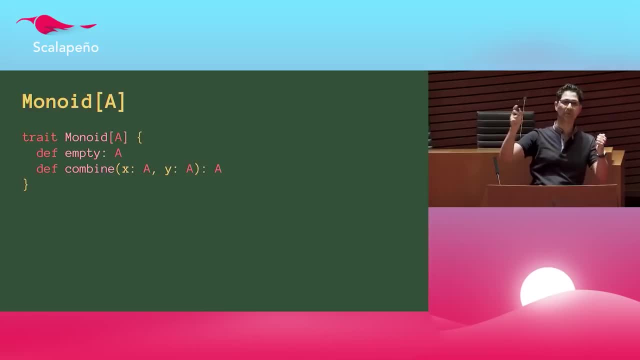 You see, the combined method is exactly the same thing: right Takes two of the same, gives you back one of the same. It's the same trait. Also, it has an empty. We will need that later. But basically for the plus right, for ints, the empty would be zero, right. 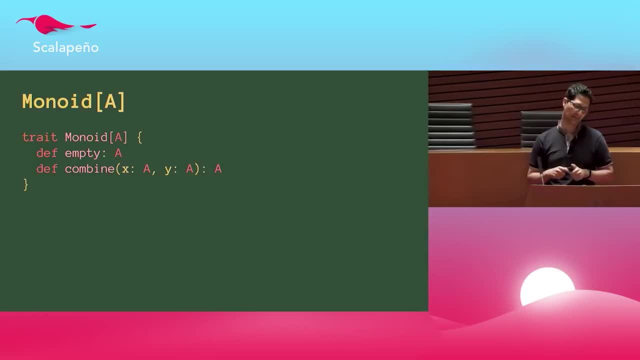 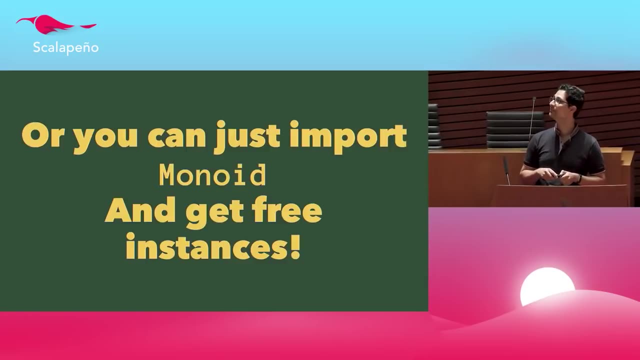 You want one plus zero, equal one, So you need this. So great. But you know what? Well, you don't have to know this stuff and you don't have to discover it, You can just import them. That's something that is extremely powerful, right? 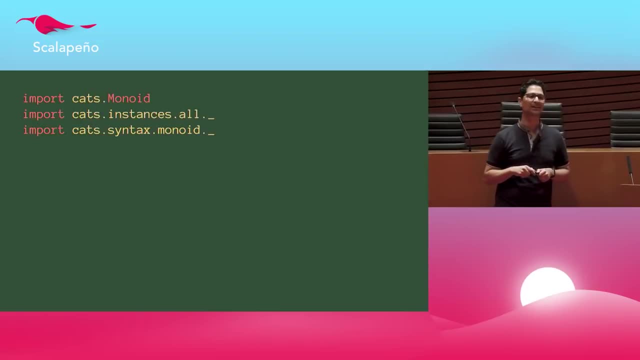 You can do that. You can import monoid from cats or from ScalaZ. You can also import the instances, right? You remember I wrote them right for ints, for strings. Well, you don't have to do that anymore. 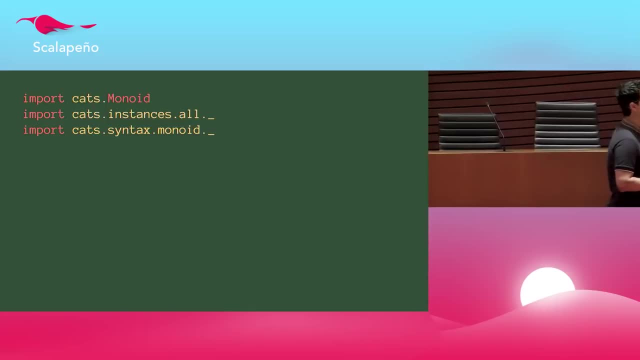 You just get it for free from the library And think about it, right, Think about how powerful this thing is. When you wrote design pattern, everybody would go to the book and would implement it its own way. There is no libraries for design patterns. 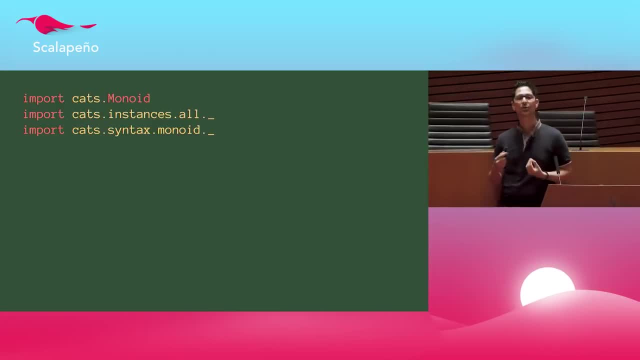 Just does not exist Here. not only you have the abstract interfaces, you also have the instances. Someone very smart wrote this code for you. You just have to take it and to use it. Thank you, Use it right. So if I import this stuff, I can do the same thing. 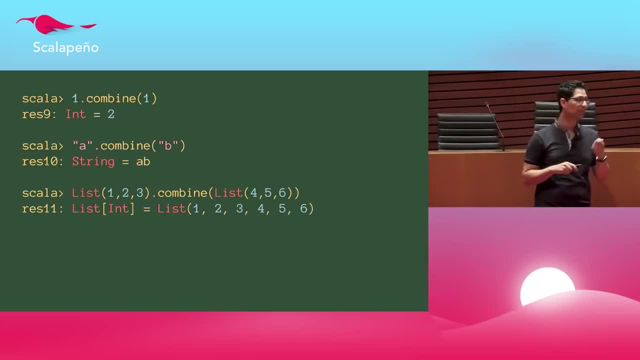 I get this magical combine method on one. On the value itself, I get this combine method. I can just use it. one combine one, two. Same thing on string. I did not have to write any code. This thing came for free. 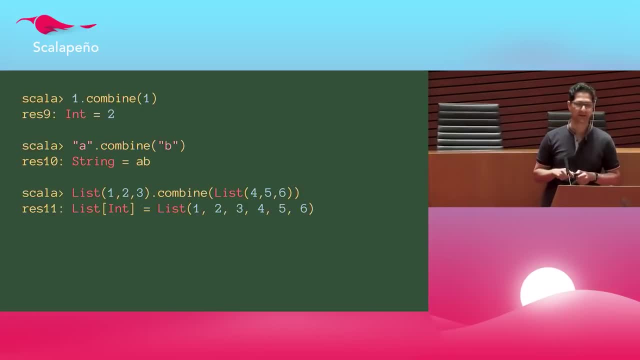 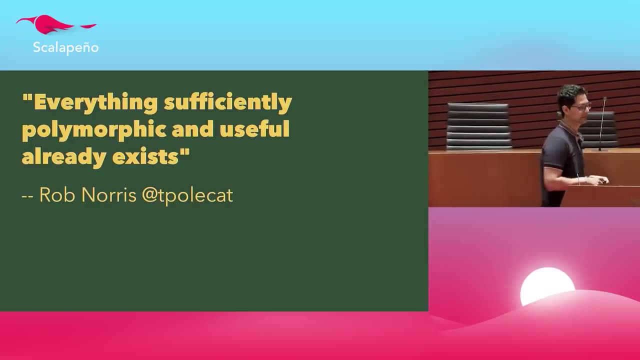 Write same thing for list One, two, three, four, five, six. This thing is great And of course that's one path. Okay, That's one pattern, But, as Rob Norris would say, everything sufficiently polymorphic and useful already exists. 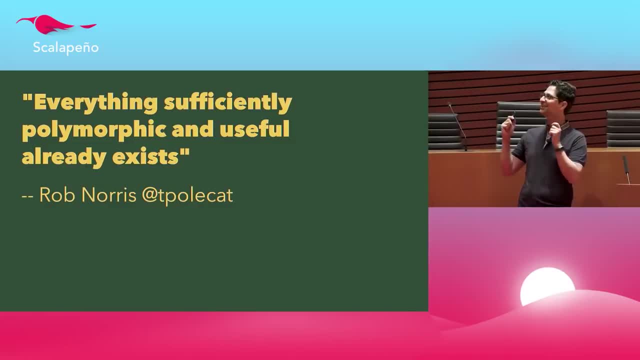 What does it mean? It means everybody that worked on these patterns, right, they already discovered for you. Okay, There is a big community out there that worked on those already and just supplied this stuff for you in these libraries. You just have to look up the documentation. 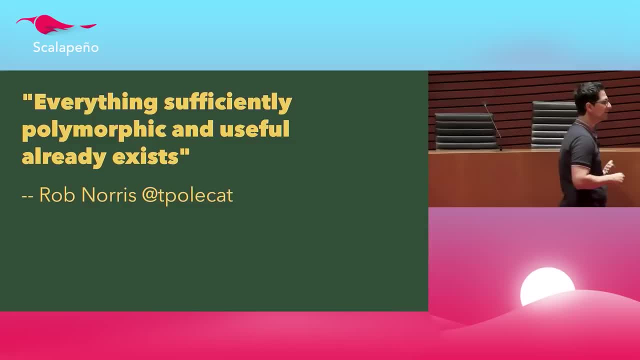 Take what you need And put it in your project. That's something that is very powerful, That does not exist in the old world. These design patterns don't have that. You don't have these libraries with implementation to use and you can just go and take what you. 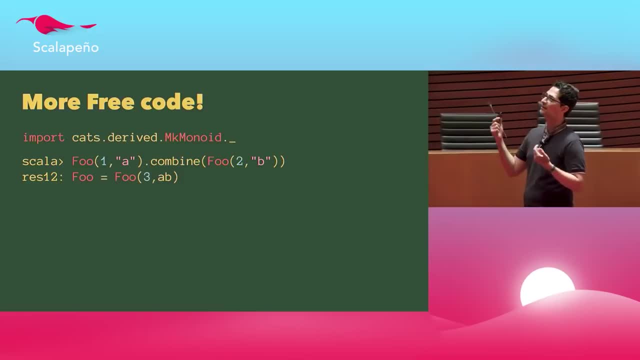 need, Also because these patterns are so common. right, this monoid. there is a huge ecosystem building on top of these libraries, All these type classes. Well, You can also get. you see, this foo class that we defined before. 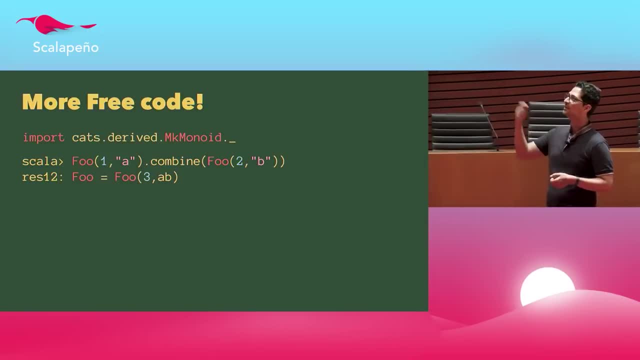 And I had to write manually the implementation. If I want, I can use this library called kittens. I just import it and it will magically figure out what is my monoid instance. It will give you magically this combined method for free Right. 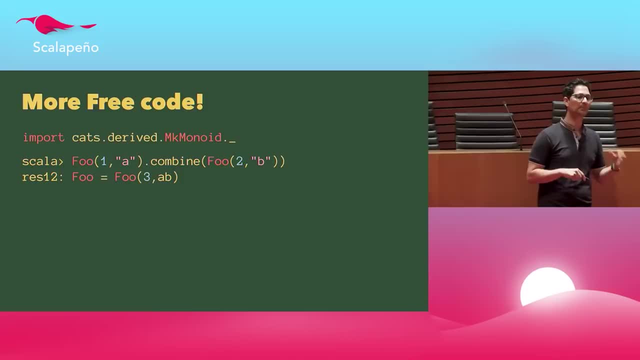 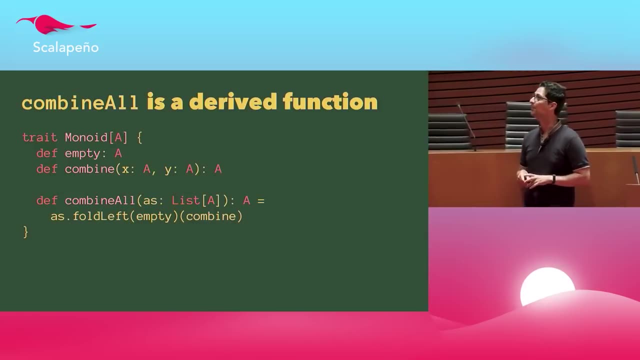 That's very powerful. All these libraries work with this functional pattern, So you get all this stuff for free. Okay, And this is an example, right, you could have what's great about type classes. it's not only that you get this free thing right, this combined, you also get a lot of what's. 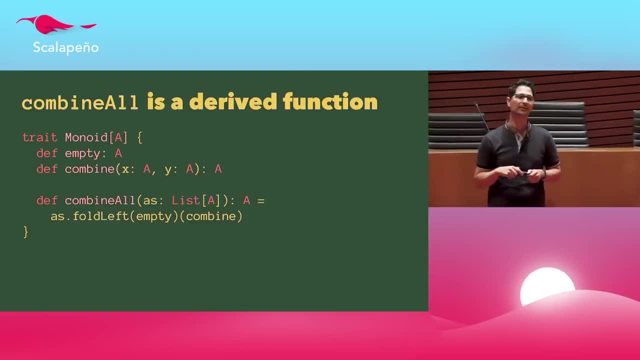 called a derived function. So let's take a look at our monoid again. The combined method that we discovered is called the function, the definitive function. right, It's defining the type class, But we also have the derived function, We also have the monoid function. 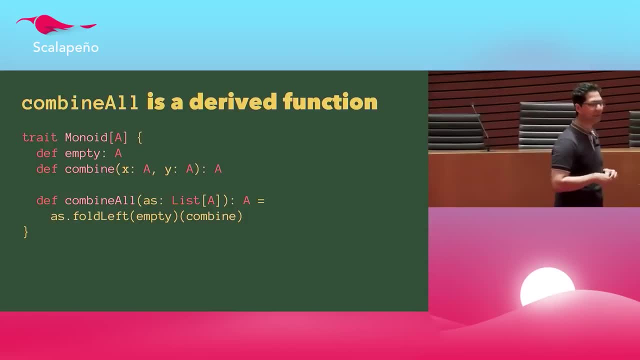 Right, We have the derived function, And this derived function here is, for example: combine all This stuff you also get for free, And that's a very interesting. I just want to show you the implementation. You don't have to implement it right, because you get it for free. 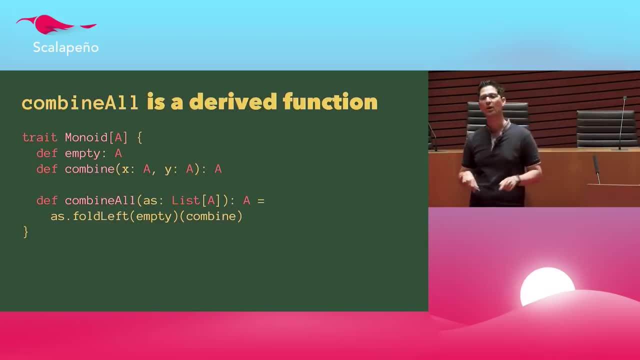 But that's the way to implement it. Think about parametricity, what we talked about before. The way. how many ways could you implement this? combine all function? How many ways? Well, not so many, Right, If you know you have to use this, empty and combine. look at this function. 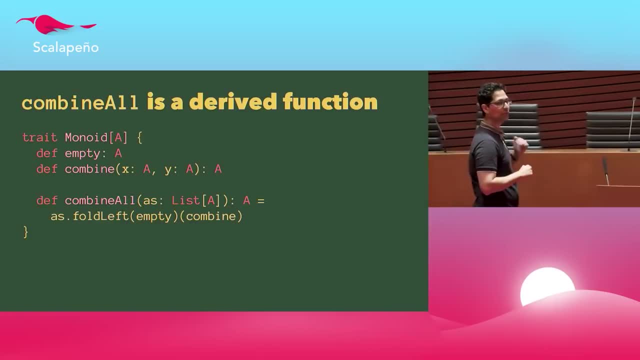 It's only defined in terms of these two abstract methods, right about empty and combine. You know you have to use them. You know you get a lot of inputs, So you know and you have to get one. So there is only one thing you can do is to take all these values and hold them. 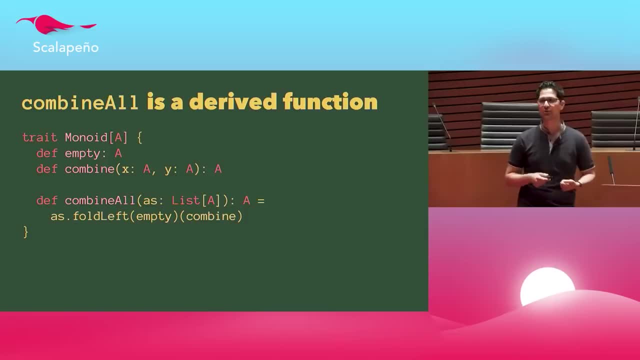 That's it. To write this function is so easy because you don't have so many options. That's it. To write this function is so easy because you don't have so many options, That's it. That's parametricity in action. 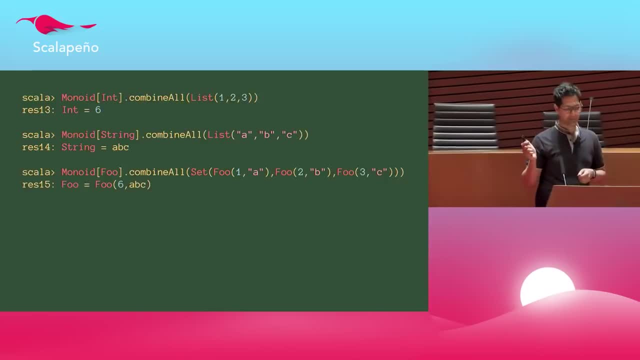 Right there. So you can just import this stuff and you get this combine all for free. So you can just import this stuff and you get this combine all for free Right Now. I can combine lists right. I can give you one to three. 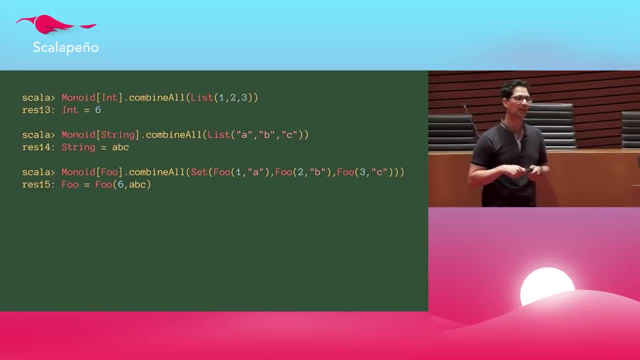 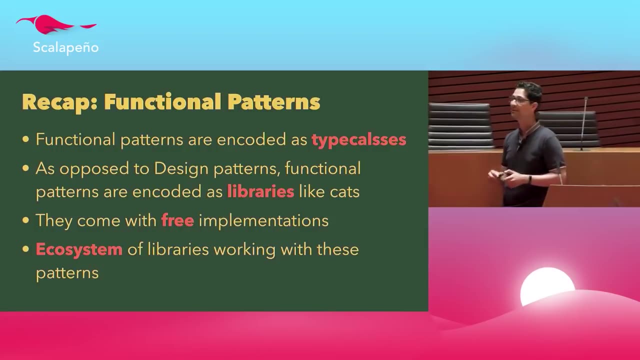 I would get six ABC. I would get ABC And foos, And it works right. So let's recap quickly about this functional pattern. How do you encode legs, functional patterns? Well, you use type classes. These type classes have parametric function and 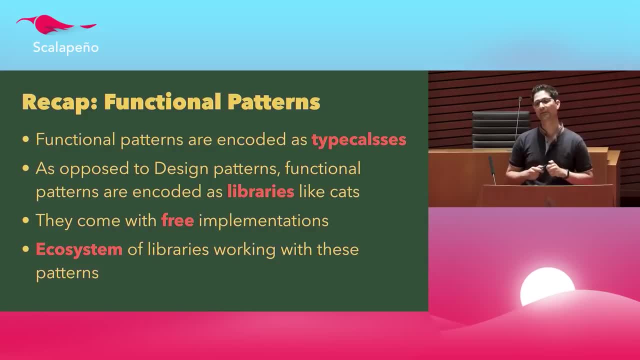 also, the way to implement these type classes would be to write instances. We saw that you can use cats or ScalaZ and import it directly into your codebase, and you don't even have to write your own instances. This thing will give it for free. Also, we saw that we have all these. 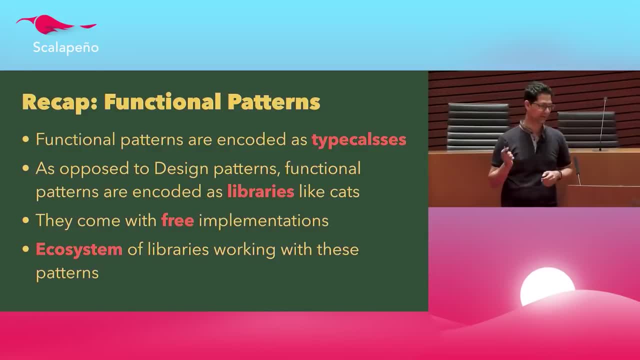 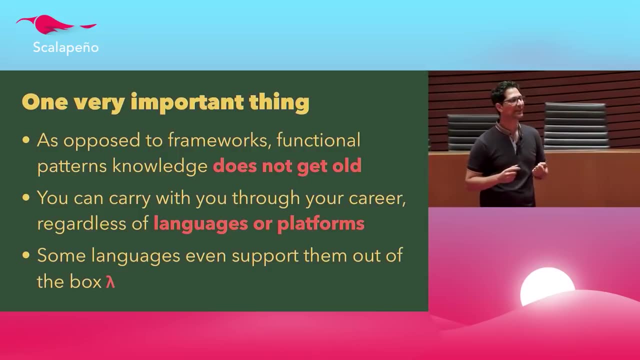 libraries that build on top of all these functional patterns. And something very important: right All this knowledge, all this functional knowledge, you keep it with you, As opposed to Spring or Ivernet or whatever framework. this thing does not get old. right? All these patterns, the way to. 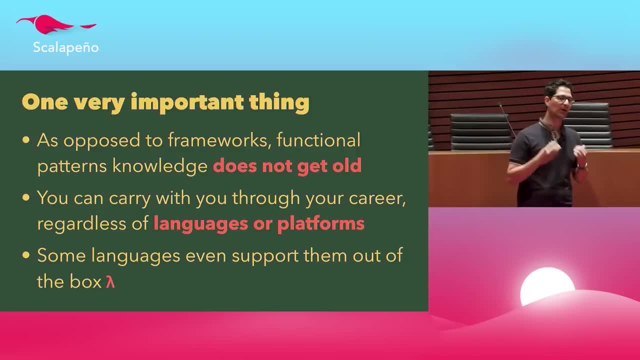 encode functions. well, you can use it for a lot of things. So you can use it for a lot of things. These things is forever. Whatever language you use, framework, these things stay with you right Throughout your career. you grow into it And you don't have to think each time when you move to a 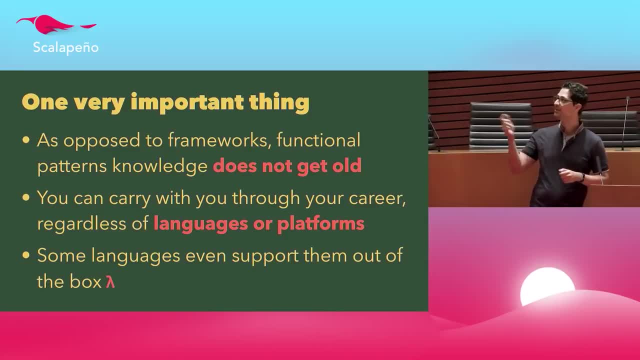 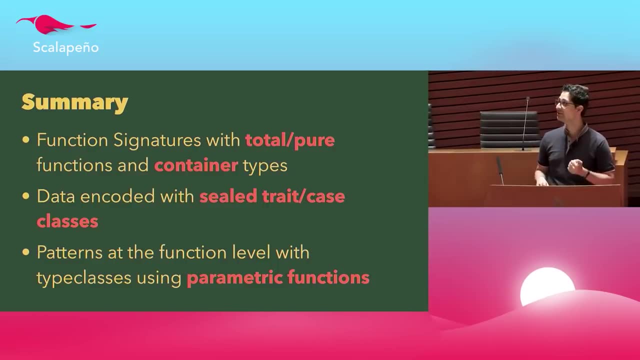 new team. oh, I need to learn this. I need to learn that. Well, this stuff is universal. So let's do a quick summary. We talked about function signatures. You can use total functions, pure functions and container functions. Now you can use any of these. All these functions are in this and this. 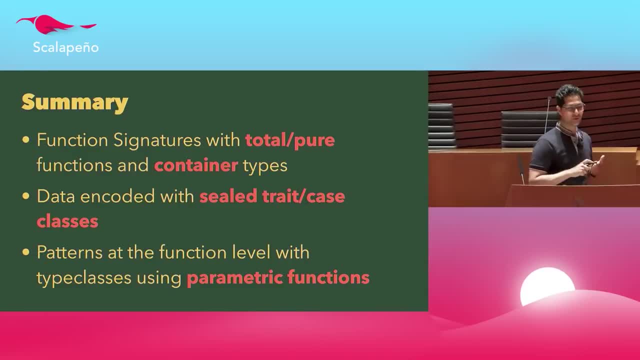 container types to write great function signatures so you don't have to think about what is the implementation, The mental stack. again, you want it free of clutter. We talked about ADTs, right about data and how to encode data in a way.